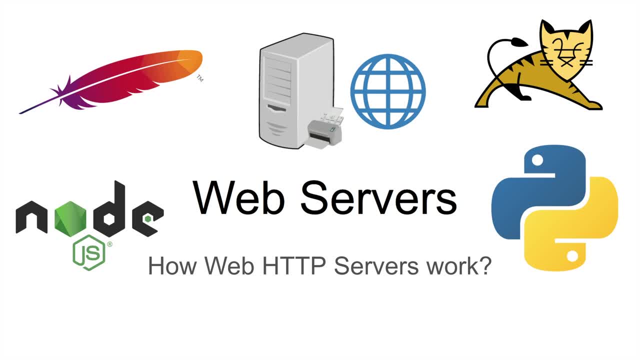 If you're interested in that kind of things, hit that subscribe button and hit that bell icon so you can get notified whenever I upload a video. That's it. Let's just jump into this video, guys. All right, We're going to jump into some. hopefully go through this theoretical part so we can show you some cool-ish stuff. 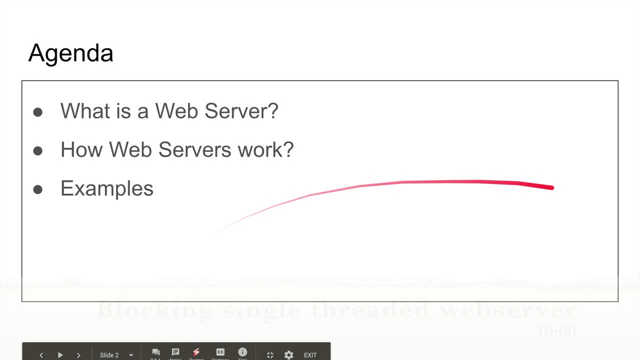 And I'm going to add some jump codes here. You're going to see it here, so you can just jump to your favorite part of this video. All right, We're going to talk about what is a web server in this agenda. We're going to talk about how web servers work. 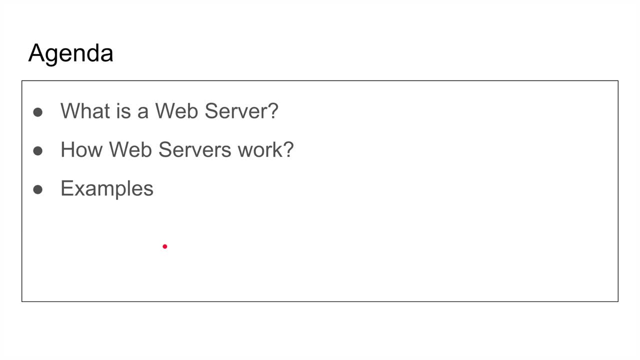 And we're going to show you the examples. right, This is our agenda for this video. okay, What is a web server? It is a software, essentially, that serves web content period. okay, Define what web content It could be: your HTML pages: 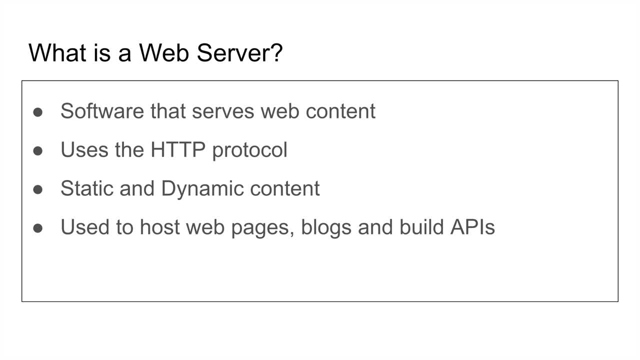 It could be just images, PDF, right. Anything that can live as a web and transfer it as a web content is defined as web content. okay, Your API could be web content, right, Your JSON document is a web content, okay. 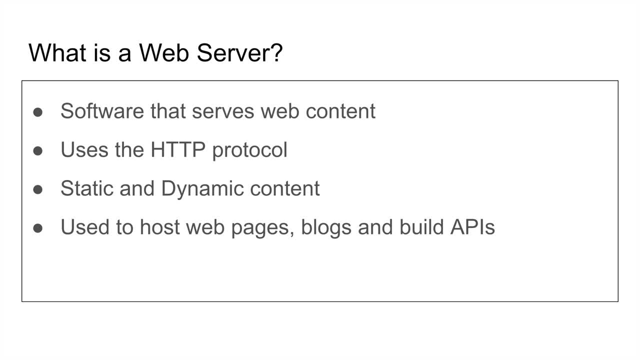 Anything that's sent back, taxed right, can be web content. That's the definition of that, okay, And it's consumed by clients. who knows how to consume it? It knows how to consume web content. okay, Let's talk more about that. 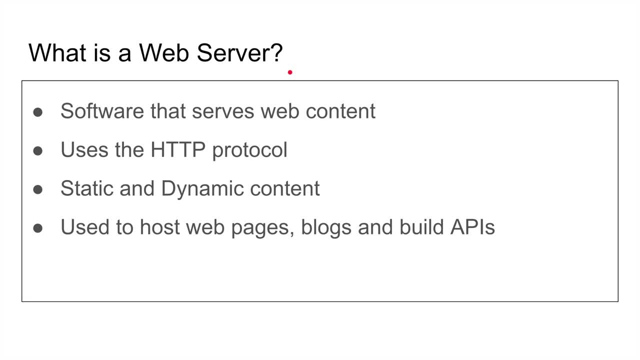 That's why it uses the HTTP protocol. And guess what? We have made a video about the HTTP protocol. I'm going to make it a reference here. So if you want a deep dive into what HTTP exactly, exactly, exactly is, with examples, go watch that video. 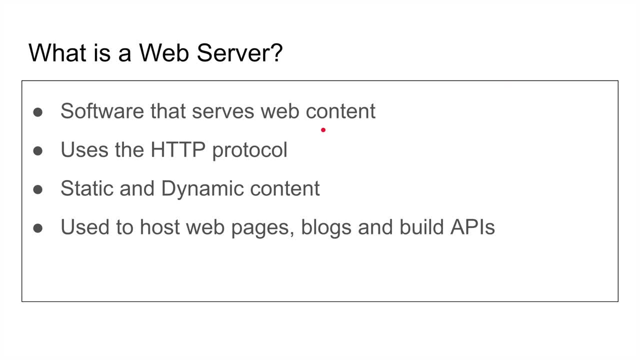 I'm going to reference it here, But essentially it's the hypertext transfer protocol. It was designed and there's different versions, different semantics, right, But we are now in HTTP 2.. HTTP 3 is coming. HTTP 1.1 has been living for almost 20 years. 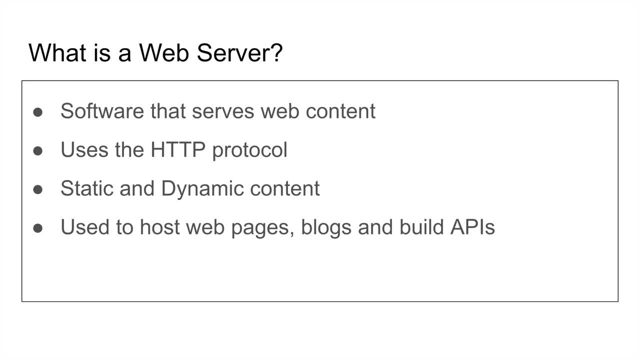 And essentially this is what the web runs on. okay, And that's what you say, like HTTP slash. slash, That's you're using HTTP protocol. okay, If you want to learn more about it, go there And all right. static versus dynamic content. 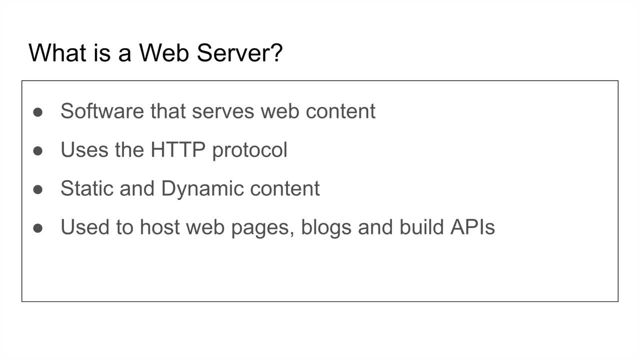 So what does that mean? okay, If you're, like me, born a millennial, born in 1983 or a little bit earlier, a little bit later. if you're, like me, born a millennial, born in 1983 or a little bit earlier, a little bit later. 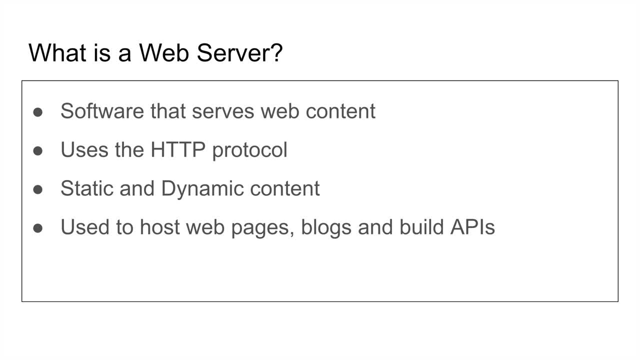 after that you will remember the early days of the web, where those flashy marquee text and the moving stuff, where the web was essentially just: you consume stuff. You cannot really change anything in the web as a user, You can just consume. It's a static content. 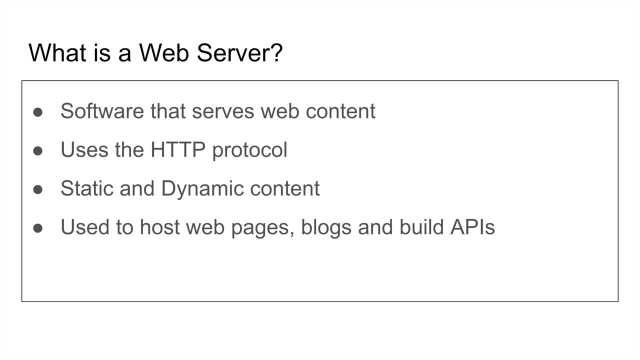 It's just a bunch of static content, HTML pages, right, Most of the run on Apache, by the way. All right, So that's like the state of the art in the 90s, if you remember. Okay, so all these flashy images. 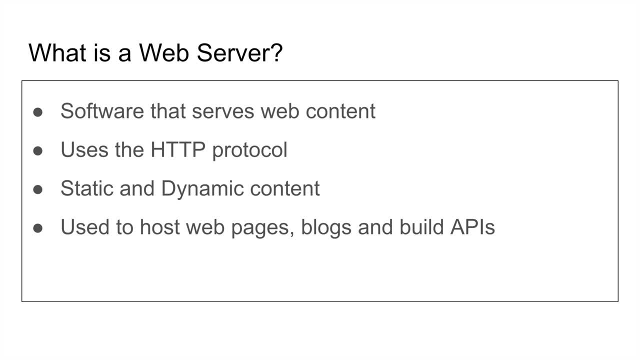 And essentially static content is like indexhtml, index pages, HTML pages, PDF images, CSS right, I don't know if the CSS existed in the 90s or not. JavaScript files are also considered as static files, which is funny because it's actually code. 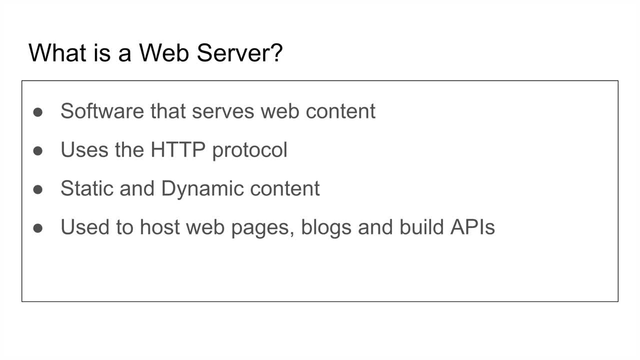 But it is Nevertheless. it's a static file. It's a file that you can download And that's it okay. And here we go, And here's the interesting part with that: Static files. So you can host a web server and you can put static files on them. 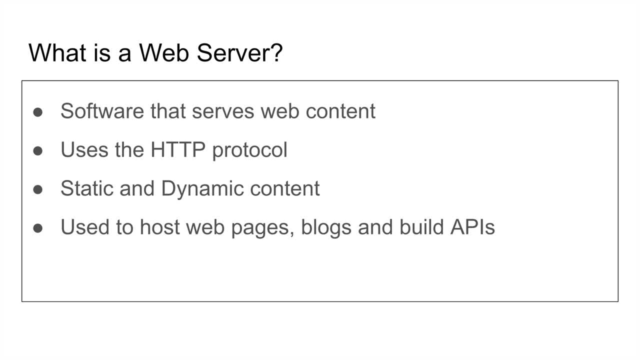 And you can serve those very easily. We can show that. Okay, That's the cool part of the web. So you author content, You paste it in a folder in your web server And then your web server will immediately generate these nice URLs for you. 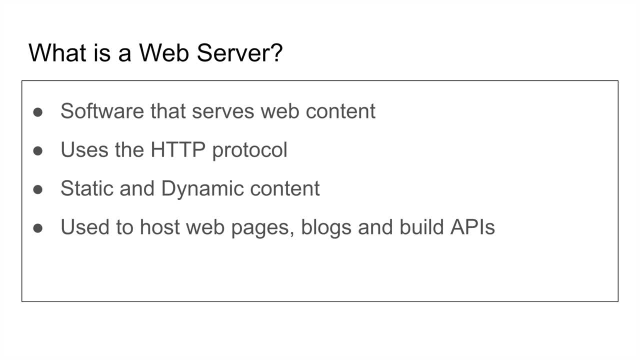 It's http, slash whatever the folder you created And then blah, You can host your pages, Which is pretty cool, right? So, people, instead of sending files by emails, you can just send people a link, URLs Or URIs. 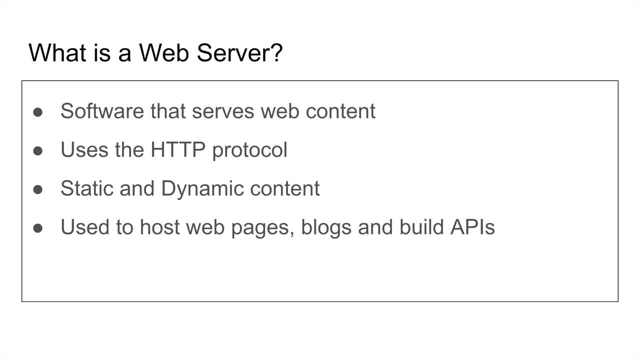 Okay, And then they will go to your content. So static files are cool because they can be cached, Because, no matter if they change, you can detect this change using ETags and caching. Okay, I'm going to reference this caching concept here if you want to learn more about it. 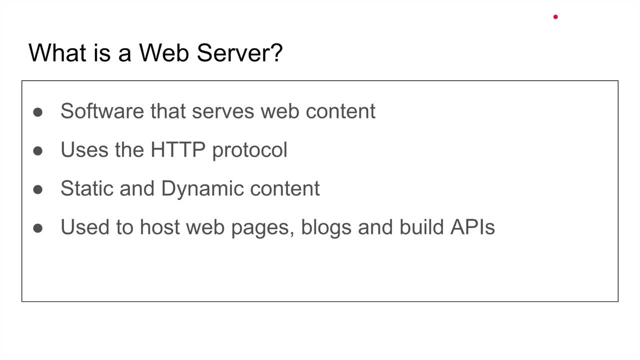 Dynamic content, on the other hand, is when things Like blog posts right. It's a query to the database and will retrieve certain results. So, based on the login user, you can get different content, different page. Facebook is an example of this right. 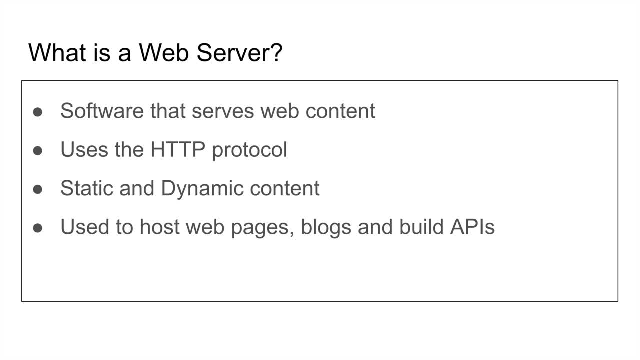 It's a dynamic. Nobody has the same web page ever, Okay, So caching this is a little bit tricky. Okay, So that dynamic content, Dynamic content, is generated as a part of a language that you write. Okay, It's a language that you write. 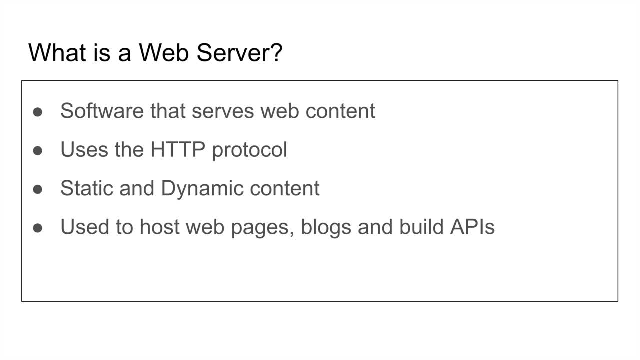 You write code in the backend that generates different page or web content based on a different context, Like it could be the user or it could be just the location. If you're coming from Asia, you're going to get a certain look and feel. 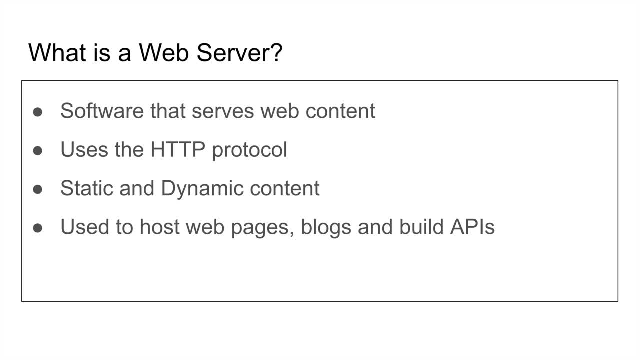 If you're coming from America, you're going to get a different look and feel. So that's the dynamic content, essentially Okay. All right, Use to host web pages. We talked about that right, So we can use to host web pages. 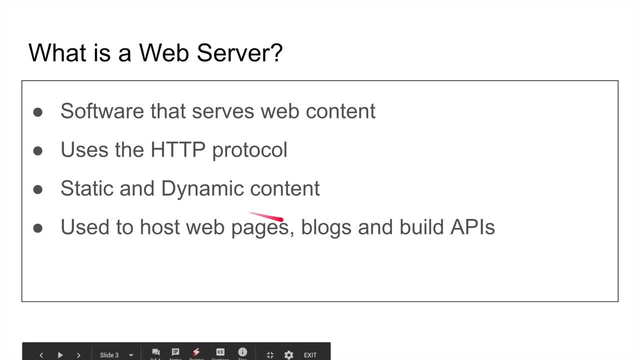 You can use. That's the 1.0 era, just web pages You used to have. You can use blogs and forums right Where you can. That's the web 2.0, right, Web 2.1.0 is everything static. 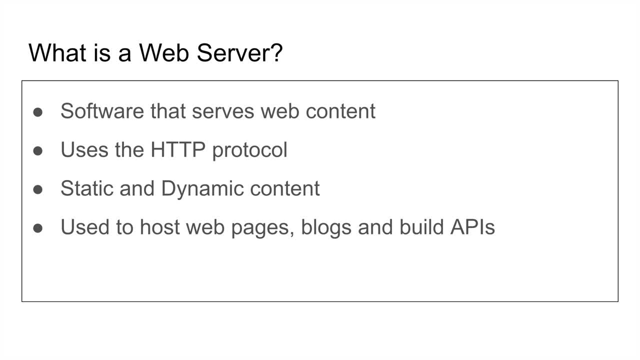 2.0 is when things started to allow users to actually interact with these pages, Like: create a comment, post it, post right, Do something And then, And then you can see these changes. So there's an interactivity between the web, right. 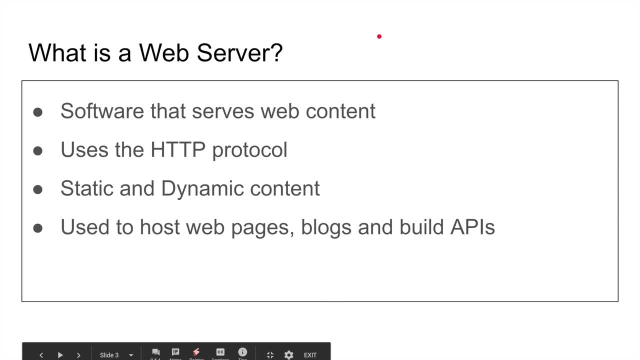 And you can also build APIs. right, We talked about APIs on this channel. I'm going to reference some videos here we made about how to build a REST API with Python. You can also check my course there- Python on the Backend- if you're interested. 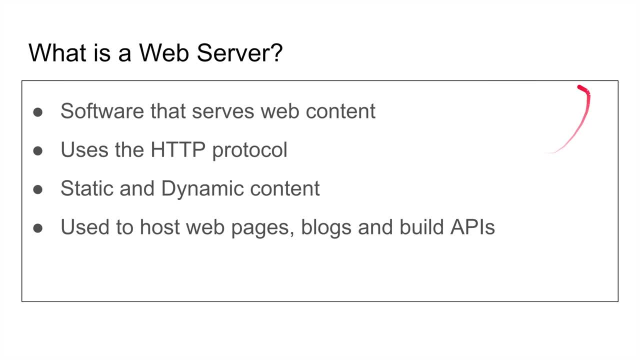 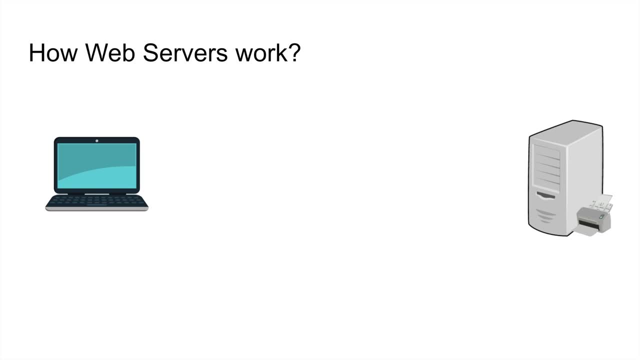 It's all about APIs and how you can write Python on the backend. A little plug there, All right. So how web servers work guys, How do those things work? I'm going to talk about concepts here that I explained before, So I'm going to gloss over them. like TCP, what TCP is right? 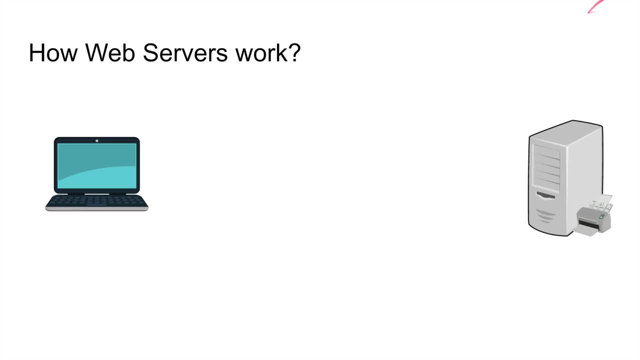 So if you want to learn more about TCP connections, check it out here. But essentially, what happens here is if a web server- This is a client- This is your web server, This is your client. It could be a laptop, It could be a mobile phone. 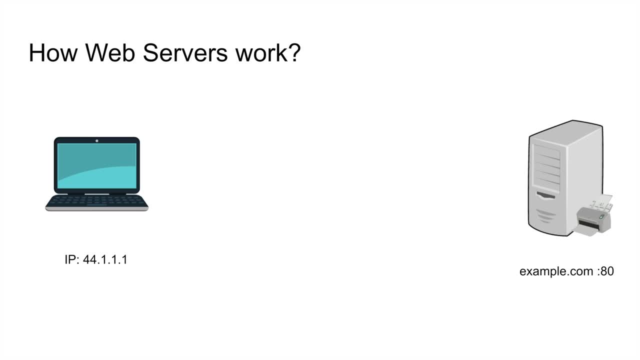 And it's requesting a page And what happens here is your IP address. have You have an IP address that cites your site? That site will have a domain name, It could have a host name And then it is running on a port. 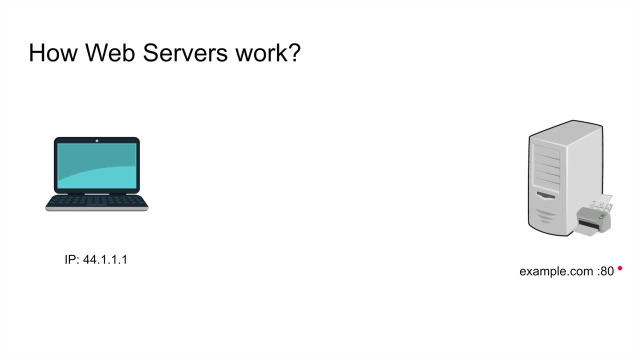 Usually this port is 80 for web servers. Okay, That's the default port, And if you don't see a port on the URL, that means it's port 80. But you can also run web server on any port you want. 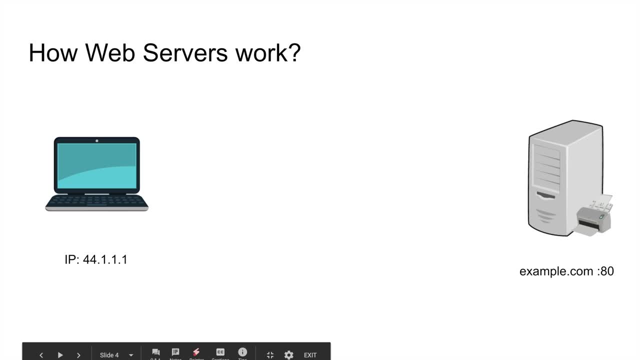 Okay, That's not, That's just the standard 84 HTTP, 4434 HTTPS. All right, So, and when you have a web server running and listening on this port, that there is a TCP socket or connection ready, right. 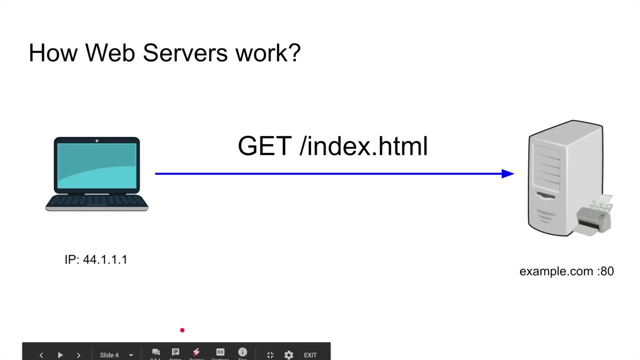 And if you make a request, let's say, get, That's the HTTP semantic we talked about. Get me the indexhtml page on the example, right, And this is a syntax for HTTP, And when you do that, the server will process that request. perhaps, maybe query the database. 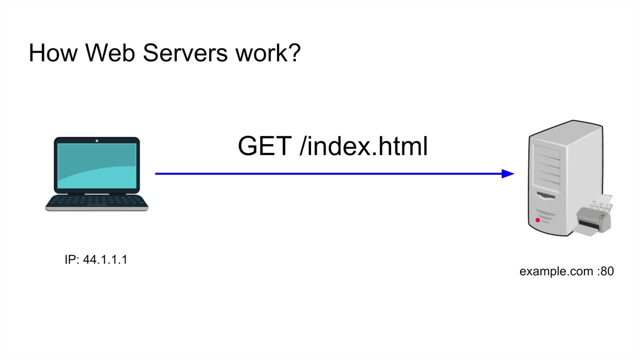 if it doesn't need to just pull it from a cache or just pull it from the directory and just serves you back the result. And then, when it sends you back, it sends you the indexhtml or whatever that HTML page And it also sends you a bunch of stuff in that response. 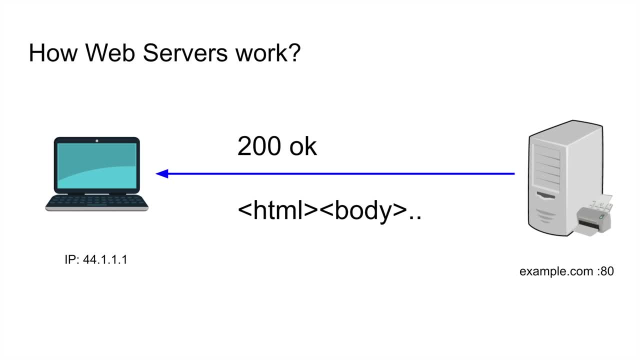 We call this the hitters and a status code, Okay, And the status code is, like you might have seen, the 200, okay, or 404, not found things like that. Right, The web servers have these HTTP codes. that, And I want to make a series about all. 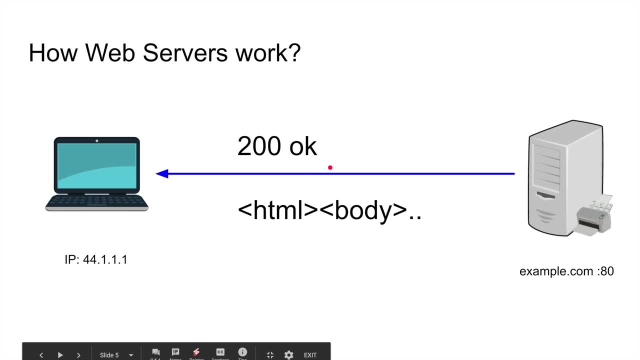 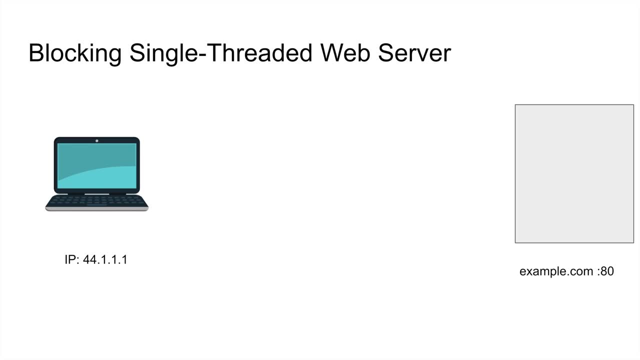 type of HTTP codes, hopefully, Okay. So that's the nutshell of that, But let's go dive deeper. for those who are daring to dive deeper into this, Okay, So another example of a web server. one example of this is what I call a blocking single threaded. 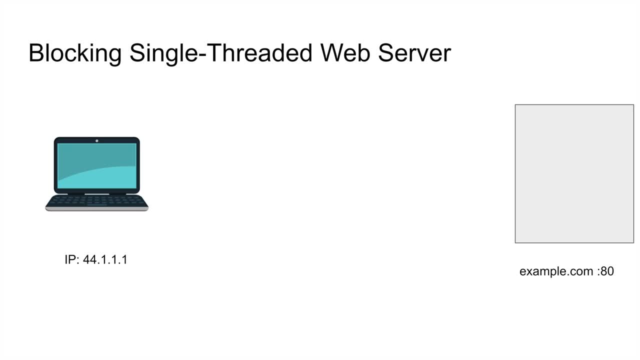 web server And I decided to explain that because it's the easiest to explain. Okay, Obviously, none of the web servers work like that. Well, I take that back. So some web servers work like that and there's benefits of that, but most web servers have. 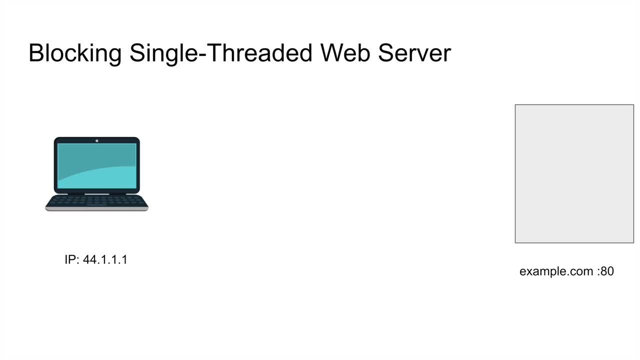 different implementation, So let's talk about it. What exactly happened when I make that get request? Okay, So this is my web server. I just made it into a box so we can draw stuff in it, Okay. And then when you first A client makes a request, whether it's a get request there. 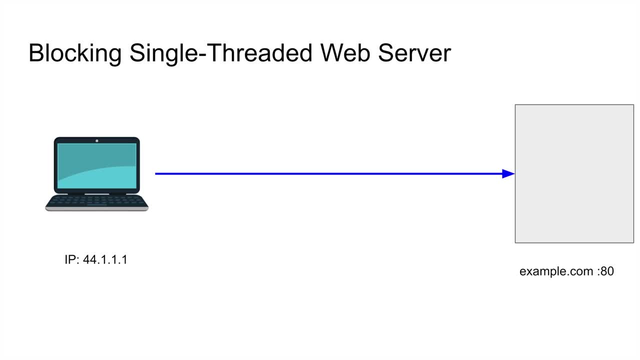 is something happening before that? Okay, The HTTP protocol runs on a transport layer called the TCP transmission control protocol. Okay, So a transmission control protocol. what it does is it establishes a two-way communication between a server or a client. Okay, 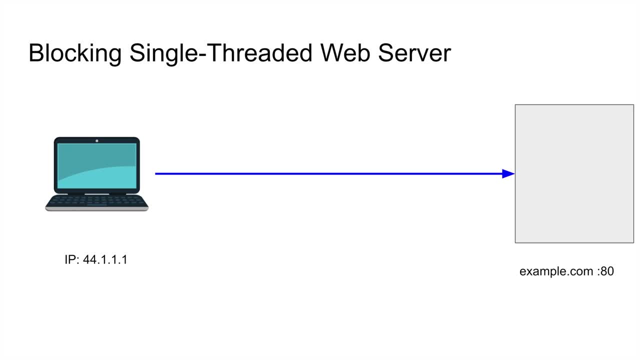 But the HTTP protocol is just a request response. So if you make a request, the first thing it does is establish this TCP connection. So this is like some handshaking going on. If there's a TLS, you need to establish the TLS. 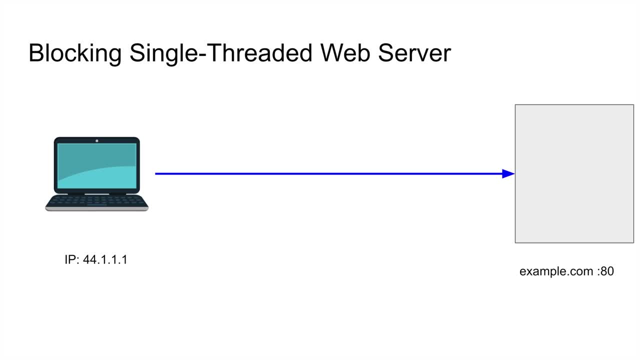 If there's a secure thing And then once you do that, the server creates in its memory- and very important here- memory. Let's focus on the word memory. Every client that connects reserves a little bit of a memory on the server. 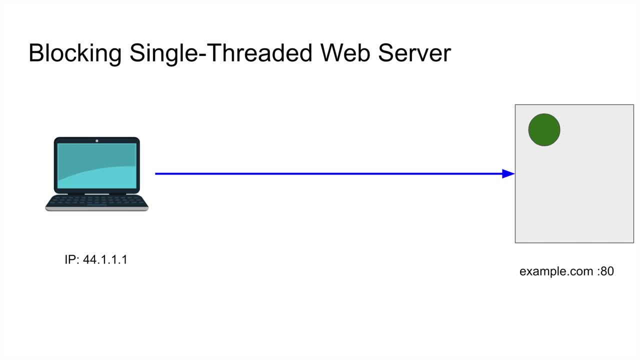 Okay, That's where things can get really tricky, Right, That's where all the attacks- denial of attack- happens because of this request, Because of this reservation of memory. Okay, Reserve a lot of memory and your server crashes. Okay, But your client connects, you reserve a little bit of a memory and this thing is called. 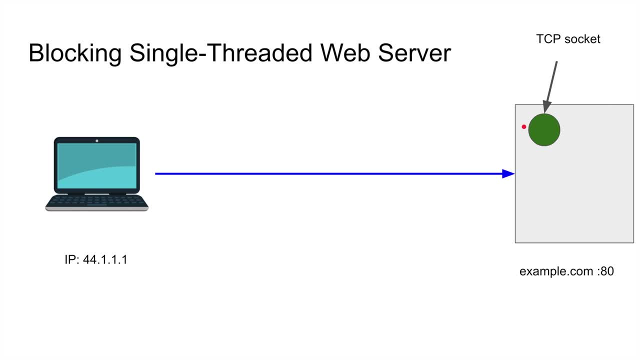 TCP socket. You reserve a socket for that client, Okay, Okay, And once you reserve a socket for that client. now you see, okay, we have one thread, one process, with one thread that is allowed to execute stuff. Okay, You can have 10 of those sockets, but they are sitting in memory. 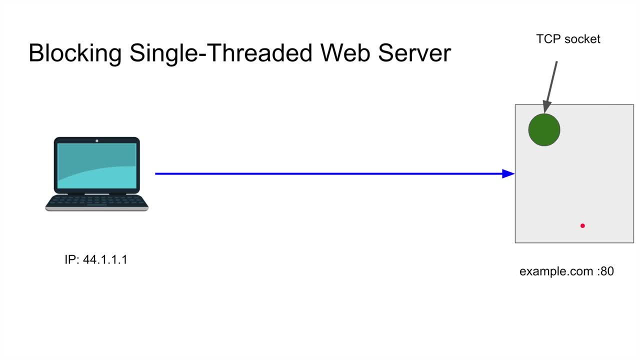 Okay, They are just idle. Okay, But your process can only execute one at a time. Okay, So let's- oh, I'm free, Your thread is free. Let's say there's a thread here, Let's start executing. 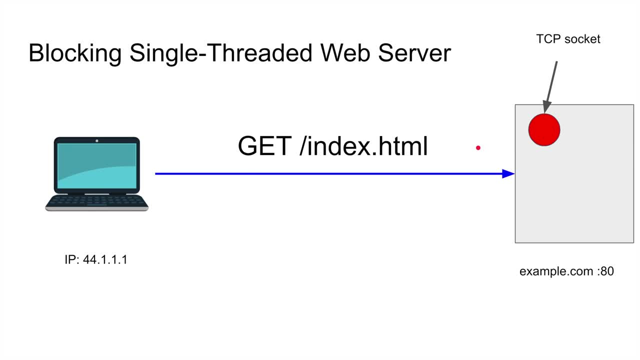 It says: okay, oh, you want me to get in this, Okay, let me go do an IO desk or whatever, Right, And then start getting busy. That thread means the socket is busy, It's doing something, That process is busy doing that. 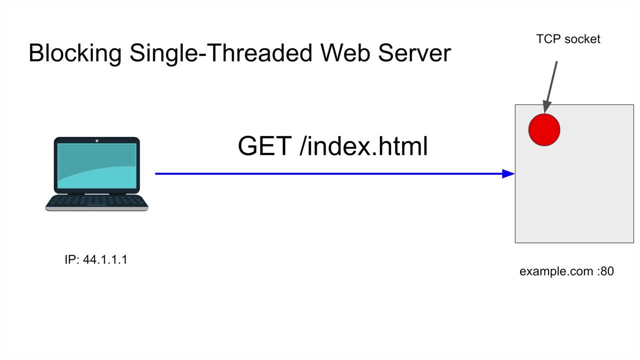 And that means that thread cannot do anything. Everything else while it's doing that. Okay, So based on that request- and that's a very simple request, but there are many requests- that actually pulls from the database or does a processing, I don't know- prime number. 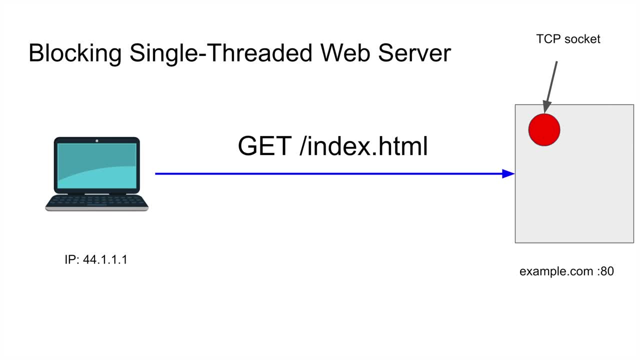 right, Do your web API thingy. Okay, And that's the tricky part, where you need to do short circuit breaking, say a circuit break and just break the circuit. if the client executes for a long time, You execute, that You release. 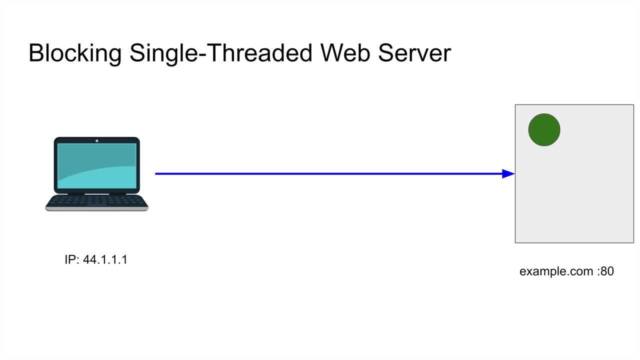 The thread is back and it's back to normal. The client got a response and we're good to go. So what happened now? Okay, So let's say I want to. the client works on another request. It can use the existing TCP connection. 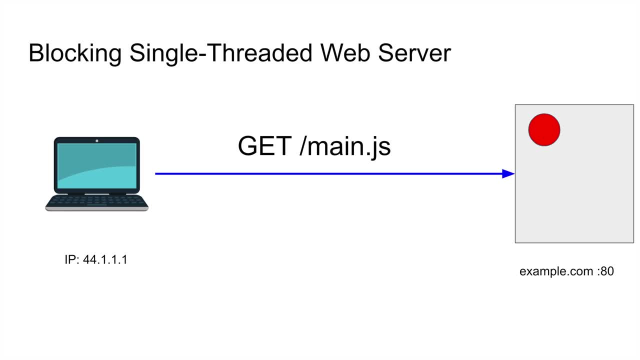 It doesn't have to create a brand new TCP connection, which is kind of fast. So having a connection TCP connection open with a server is a kind of nice thing. There's a bad thing about it, It's just you have your server. 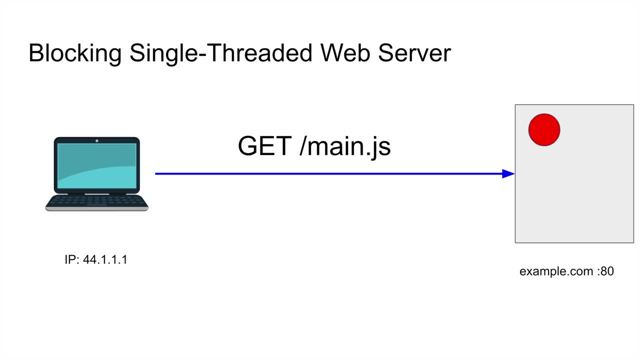 You have your reserving memory on the server. So if you have a TCP connection that is open and you're not using it, you're wasting server memory. Okay, But yeah, pros and cons of this, And we talked about the HTTP. 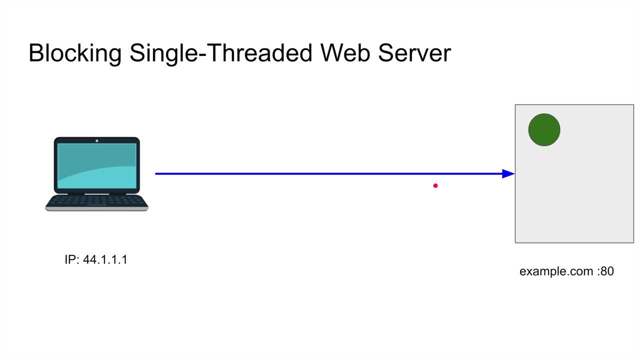 And then we go execute and then release. All right, Let's make this a little bit spicy. Let's add another client. Okay, One client makes a post request. That's the right request to the server. Okay, So I want to write something like: I want to create a new to-do list in my API. 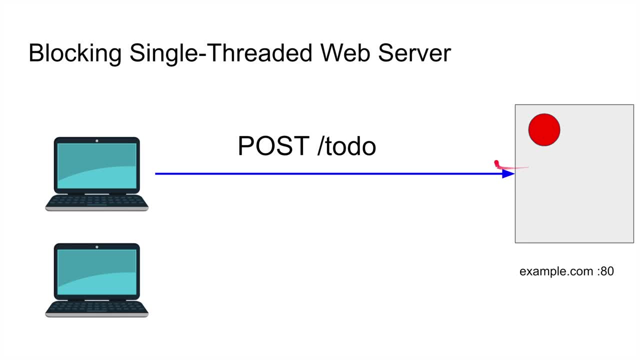 And the web server takes that and starts processing. And guess what? A poor Joe Slop here wants to connect to the web server. Okay, And the server is a little bit busy, And now the web server implementations shine. What do you do? 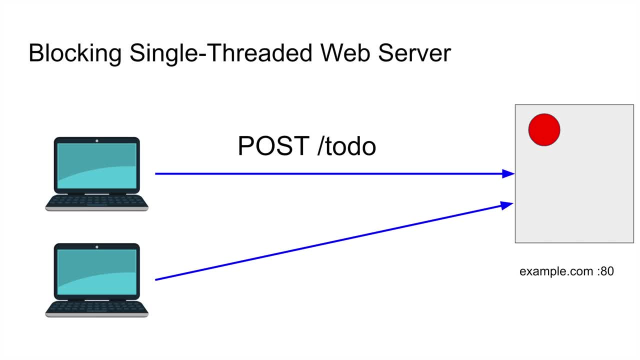 What do you do as a web server implementer? Apache does one thing, Tomcat does the same thing, All right. Nodejs does another thing, Python does another thing. You can do whatever you want, if you write your own as well. 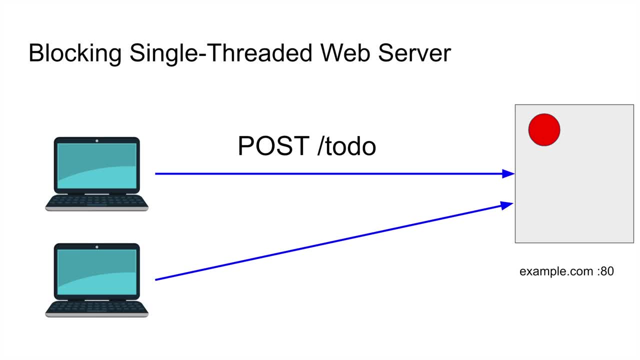 Okay, You can do whatever you want, But here's what a blocking single thread does. Okay, It creates that TCP socket for you, That's it, Just that It creates a memory for you. But guess what? Sorry, I can't serve you. 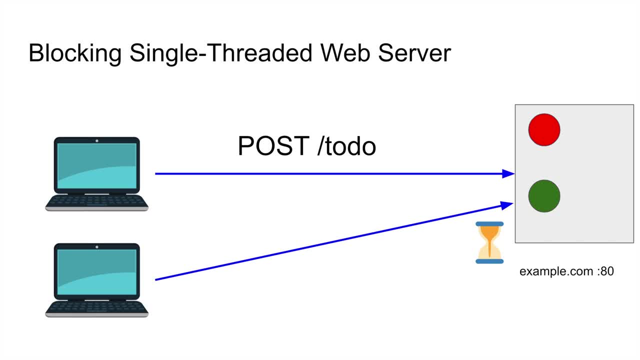 Yeah, the only thing I could do is just create that socket for you. Yeah, you have a TCP connection. Booyah, That's it. That's it, But I'm busy serving this guy now. Okay, That one thread is busy serving that. 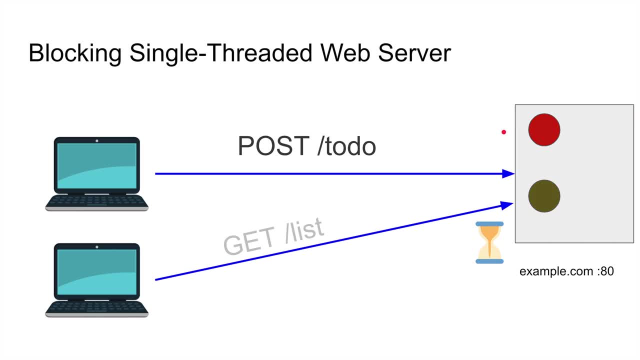 Okay, And then, once you basically done right, this guy can be served, And then you release and you're done, Okay. Some of you might say now, okay, can you just spin up another thread? Sure, That's what Apache does. 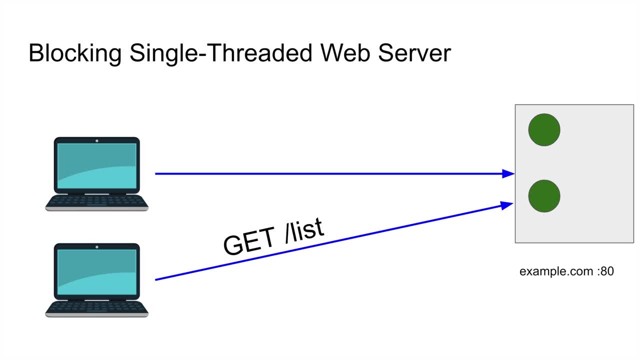 It spins up a new thread for every single request. Okay, And that's why you will see when you go to Apache or Tomcat, there is a parameter called maximum thread numbers or maximum connections. Right, How many of those do you want? 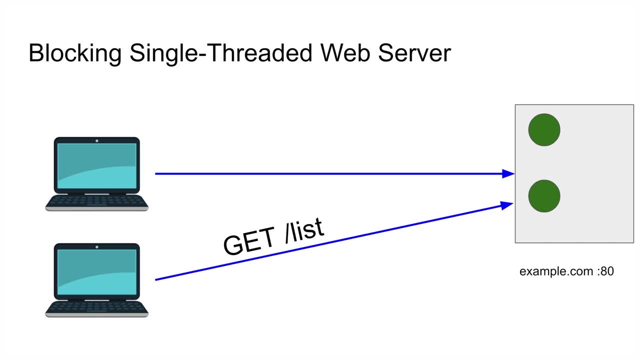 Right, I cannot just have unlimited Right. Well, you can change it to unlimited if you want, if you have unlimited memory here, But think about that when you really work with web servers. I'd like you to think about all of that stuff. 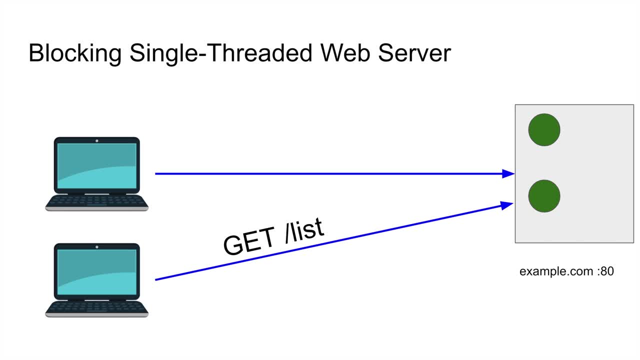 It is really interesting to know how stuff works, Especially web servers, Because we work with these As software engineers. I mean writing REST APIs. this is very critical. to understand, guys, Okay, So your implementation of how it looks like is very critical. 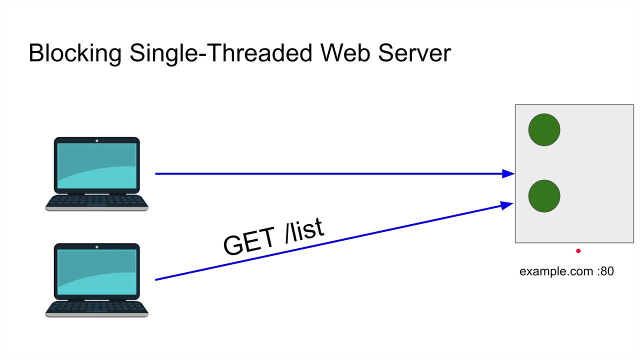 So you might be happy with a single threaded blocking, Okay. But you might say, okay, I'm going to spin multiple web servers like that, Okay, So I'm going to put them behind a load balancer And that's fine. 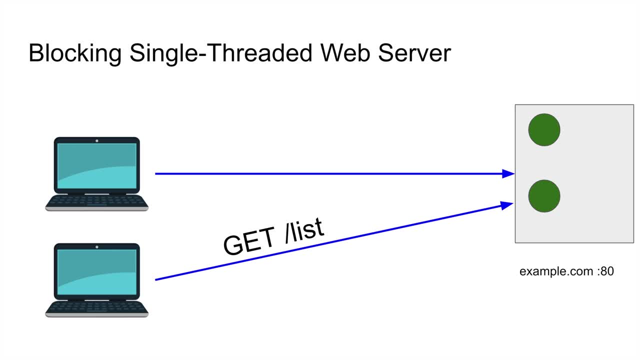 Why not, Right? I don't see anything wrong with that. There might be some limitations. Right, You can put in Docker containers. You can spin up as many containers you want off single threaded. I find this way more simple than having complex thread multi-threaded app web server. 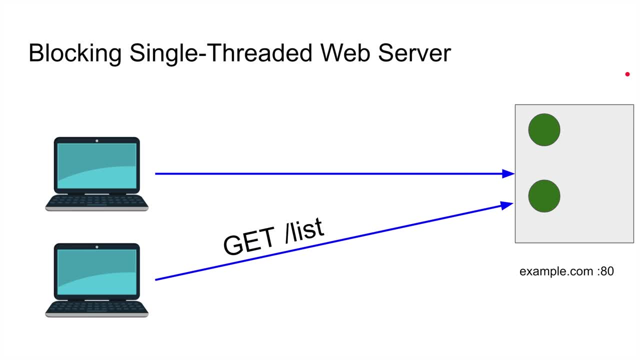 Right, Let's have a discussion in the comment section. guys, What do you think is a better way of doing things? Okay, There is no right answers or wrong answers here. Okay, People still debating this. Okay, This is set on stones. 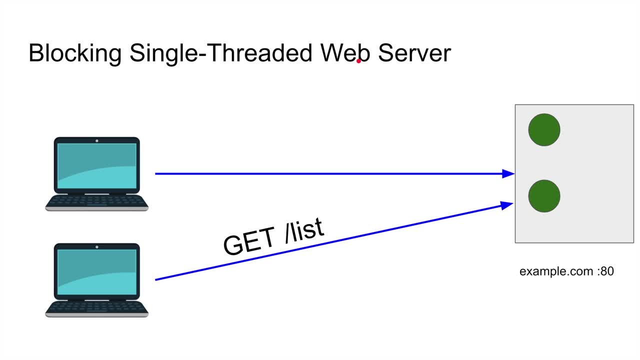 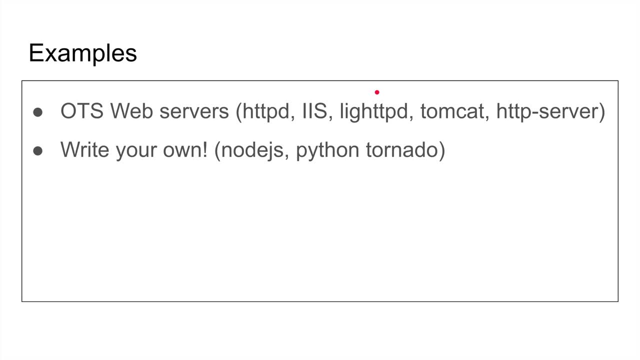 Right, Don't just absorb information, Discuss Right, Challenge everything that you read. Okay, Nobody's perfect Example, All right Example. I love this part. I love this part so much. Okay, So I did a Google search on some of the web servers. 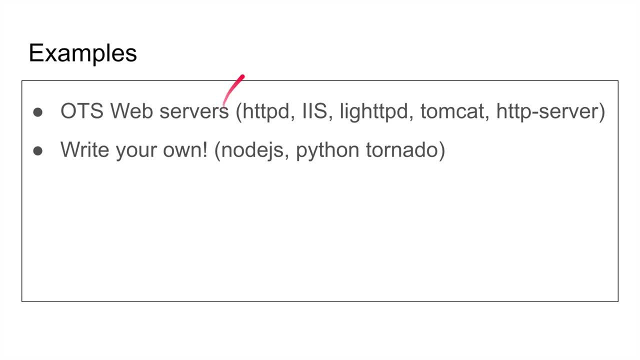 Right. The one I knew was, to be honest, I knew HTTP. I didn't know it was called HTTP. By the way, this is Apache. The other name for it is called HTTPD. I know IIS. I work with IIS most of my time. 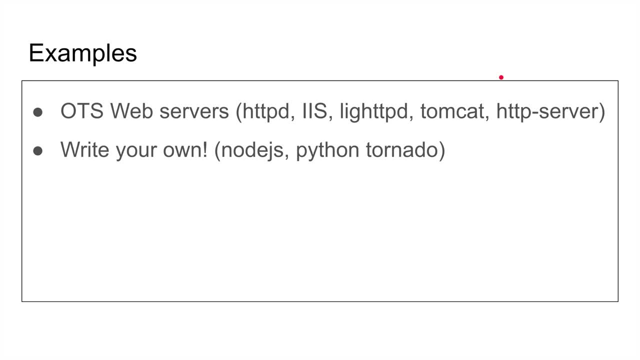 I work with Tomcat almost on a daily basis. my current job Right. I use HTTP server all the time on my YouTube videos because it's the easiest thing ever in life. Okay, Light HTTPD, which I think they force you to say lighty. 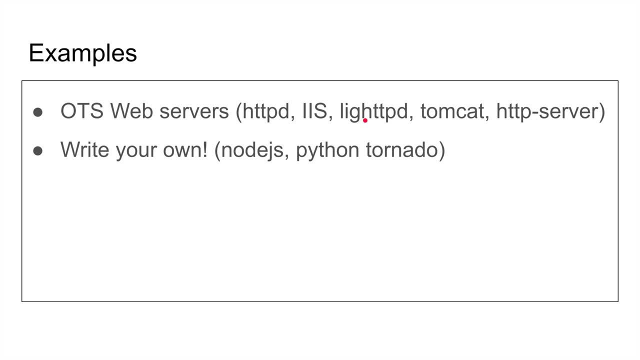 I don't know why it's called lighty. There is an H, there is a G, there is a P, there is a D. As a foreign non-English speaker, this is all wrong, by all means, You know, So write your own. 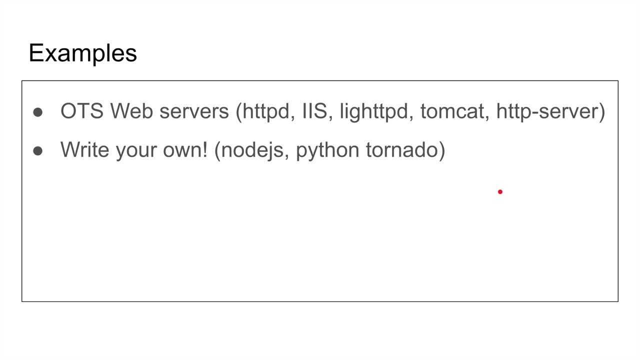 That's another way of writing, So you can use an existing web server or you can write your own. You can just use Nodejs as a framework, a web framework, or you can use Python, Tornado. So, guys, you can write your own web server as well. 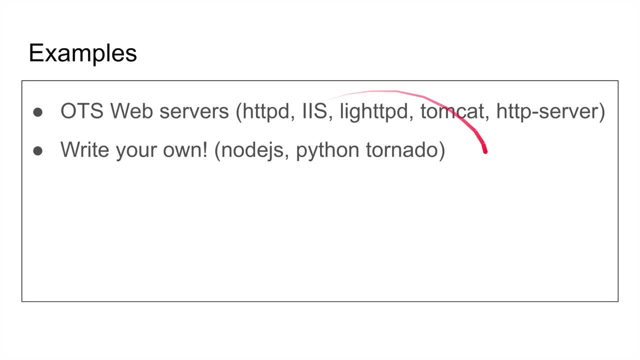 Right, And you can use Nodejs for that, You can use Python, Tornado, And that gives you the bare metal bones of things Again. it gives you how to listen to a port, It gives you how to send statuses, It gives you how- hey, there is that request and response came. 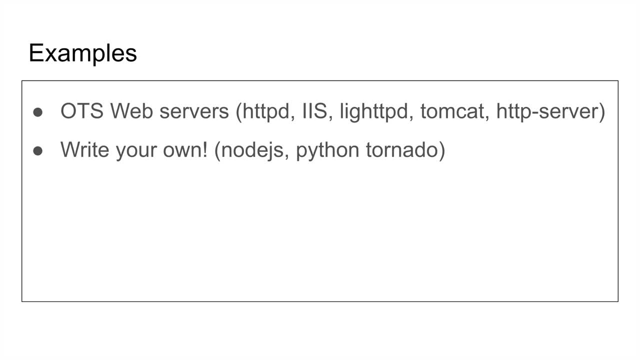 Do your thing. Okay, It can div. So it gives you essentially a blocking, single threaded okay server. But you have to write all of that stuff for yourself, Okay, So these guys does most of the work for you. If you have IIS, you can just write an ASP application. 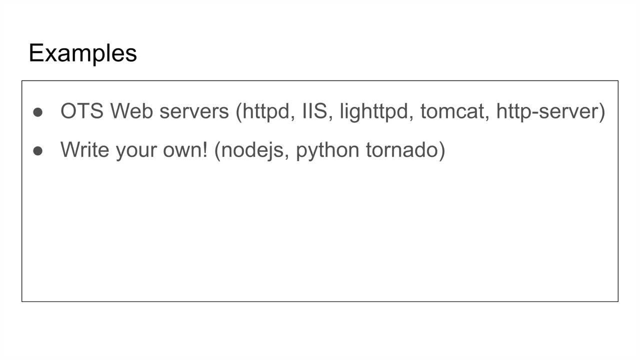 I forgot what ASP stands for ASPnet Active Server Pages. I think It says that. I think something silly like that. So yeah, for Microsoft, you can just really enable IIS and just copy ASPnet pages and then that works like that. 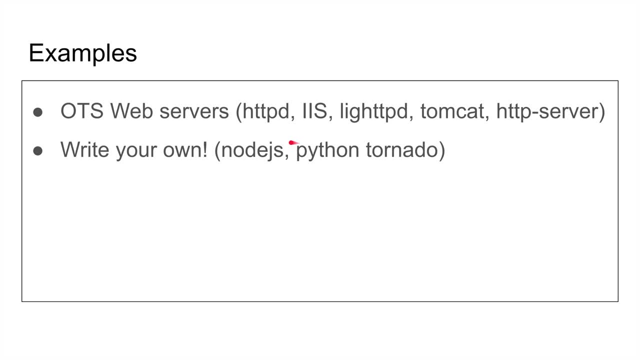 For the demo part of this, guys, I'm going to show you how to spin up Apache 2, which is HTTP D also, Okay, And we're going to show you- I'm going to show you- how to spin that in my Raspberry. 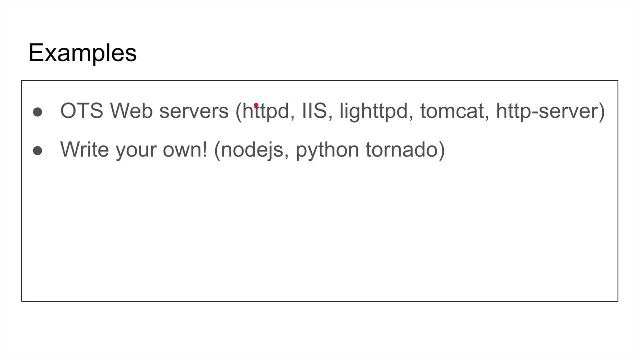 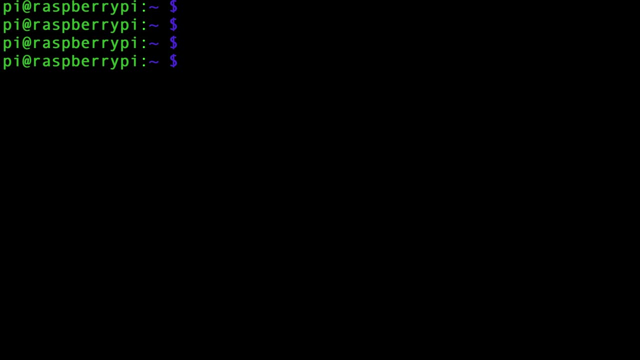 Pi, because I have Linux there. Okay, That's the easiest thing. All right, And I'm going to show you how to do your own web server using NodeJS Express. All right, guys? So here's what I want to do. 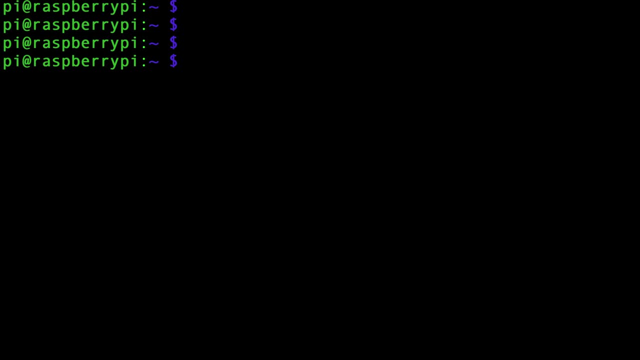 I am logged in here to my Raspberry Pi, which has a Debian distribution, and I'm going to install Apache 2, which is HTTP D, Which is the Apache web server. Okay, And this is one of those ready-made web server where you can just throw a web content at. 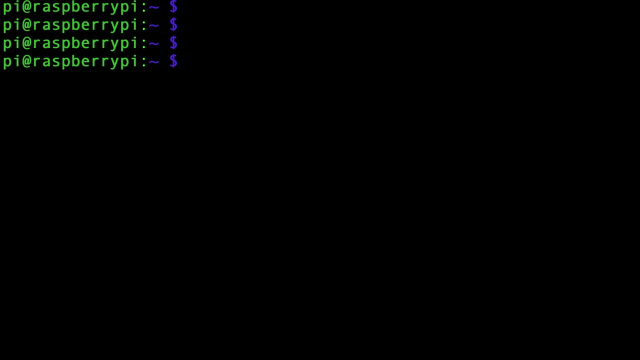 it like HTML images and it just will serve it for you. Very simple stuff, Right? And so that's the easiest way of hosting a web page, or hosting a blog or things- that, If you want to host a web page or a company website, this is the easiest thing to do. 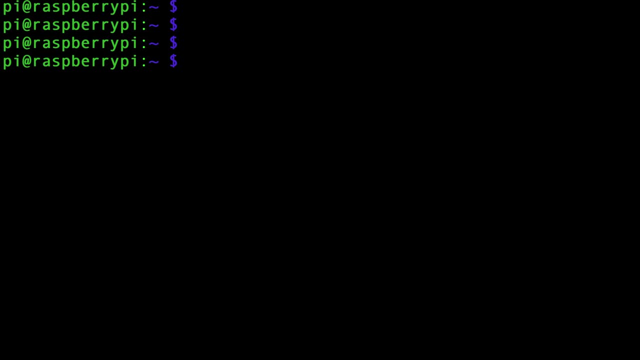 Right, So let's learn how to do that. Okay, So to do that, since I'm using Debian, I'm going to do the apt-get here: sudo, apt-get and install. It's called Apache 2 for some reason. 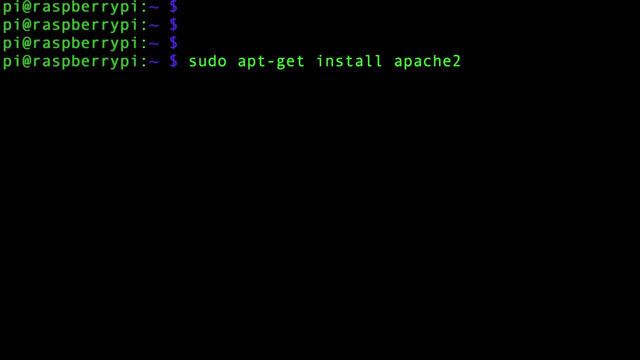 Okay, Maybe the first version sucked, so they made it another version. It's called Apache 2.. Okay, If you're using Docker, it's called HTTP D. Maybe we'll show you how to do that in Docker, So let's go ahead and install. 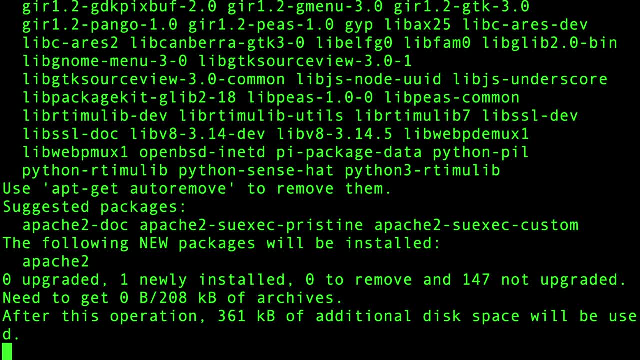 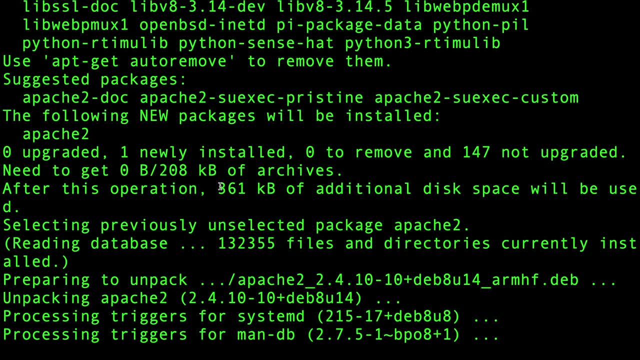 It's going to take a while. I'm going to pause the video. I'm going to show you back whenever this is done. I really can't believe that this is only 361 kilobytes, which is pretty amazing, if you ask me. 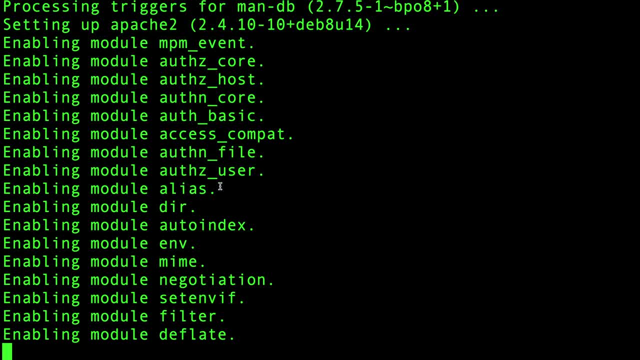 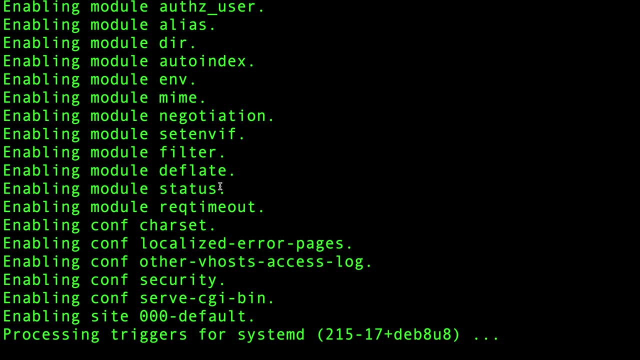 Right, This is really. It's written in C, I think, Or C I forgot Last time I checked. it's written in C, so it's a very, very small footprint, Right? Unlike Tomcat. Tomcat is written in Java and it is really heavy stuff. 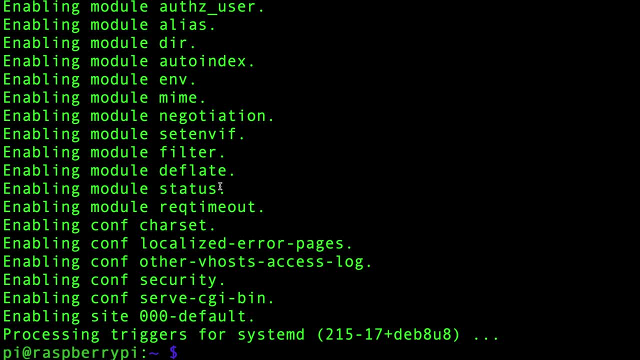 But you can do way more stuff in Tomcat, obviously. But yeah, It's done, That's it. Okay, We just installed it. Well, in your case, I have installed it before and then I uninstalled it, so you might know. 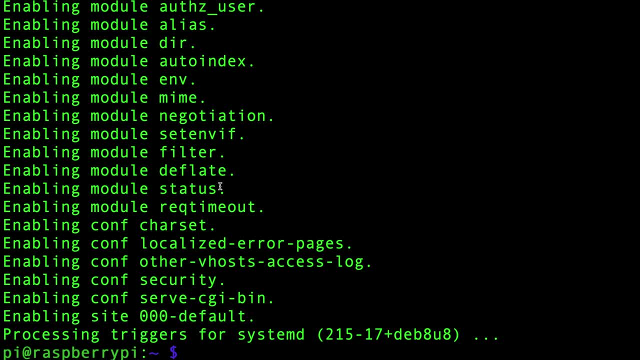 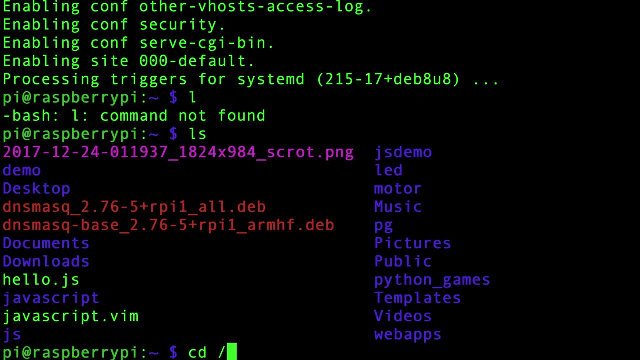 what to do. And so do apt-get update, and then so do apt-get, install Apache 2, and then you'll have it. So what do we do? Once you install it, you go to a folder called var- wwwroot, and there is a folder called HTML. 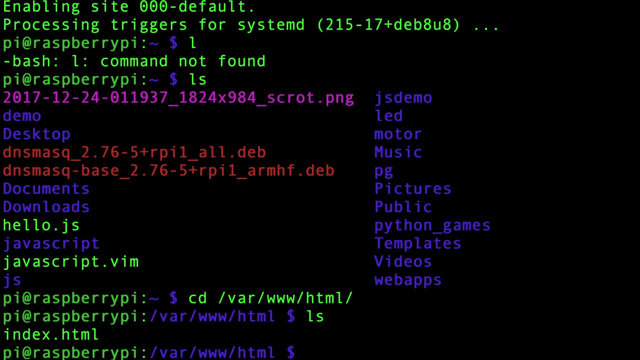 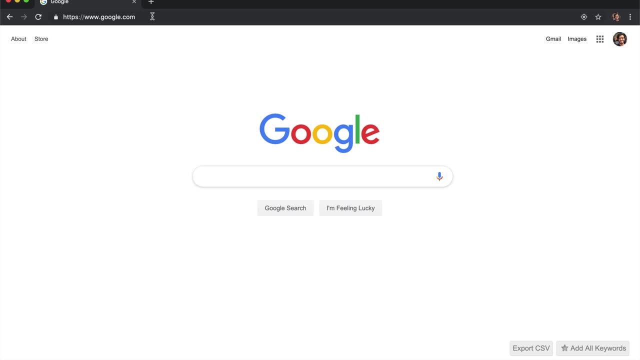 Okay, And there is literally a page called indexhtml. They give you for free to test your stuff, So let's go ahead and see if that works. All right, guys. So I am here on my Mac. My Mac and my Raspberry Pi are on the same Wi-Fi so I can access that stuff. 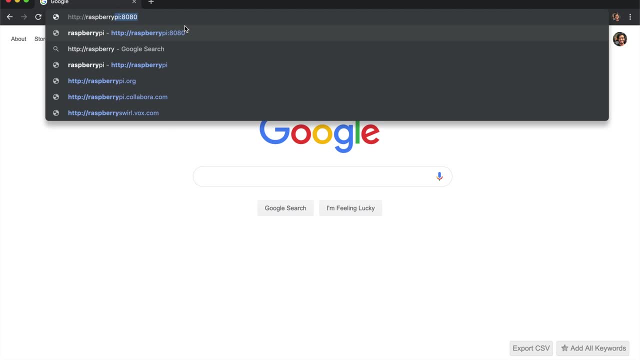 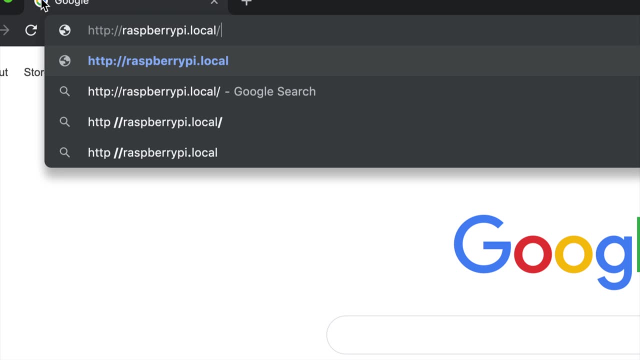 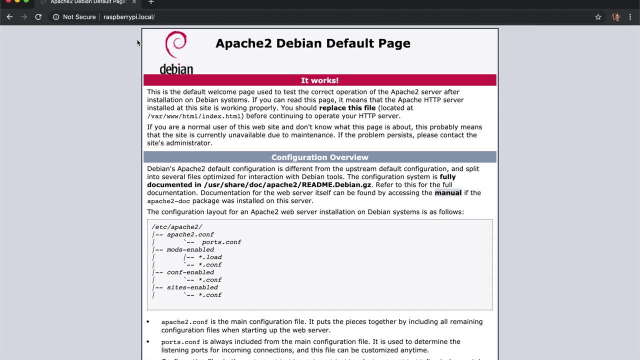 Right, So I'm going to do go wwwraspberrypylocal And by default the Apache 2 listens on port 80. So this spins up a The server on port 80 by default. Okay, So if I do that and then runs and you can see it works. 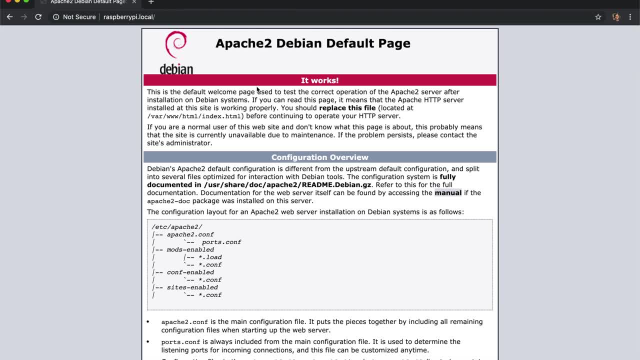 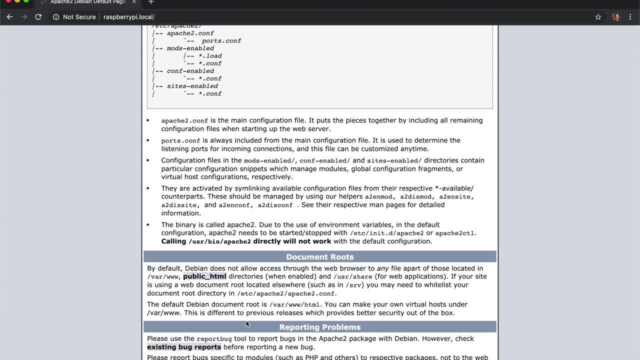 And I'm using Debian, obviously Okay. It tells you that, hey, you have your Debian distribution, But essentially it tells you what to do as well, Copy stuff in that and you get yourself a web server that can serve anything you want. 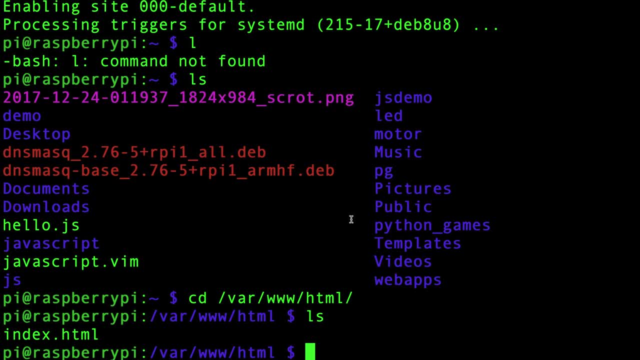 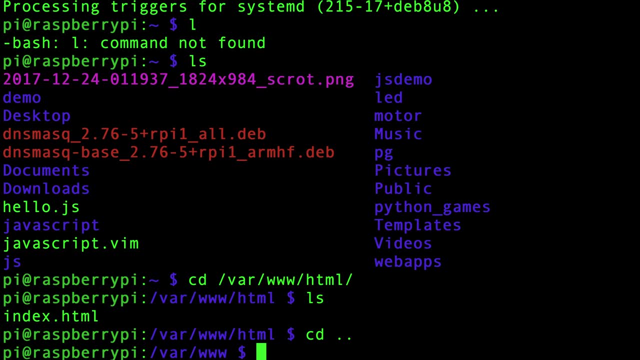 Okay. So since we guys are curious, let's do that. Okay, First of all, I'm not the owner of that thing, for some reason. So what I want to do is I want to change the owner of this thing. All right, guys. 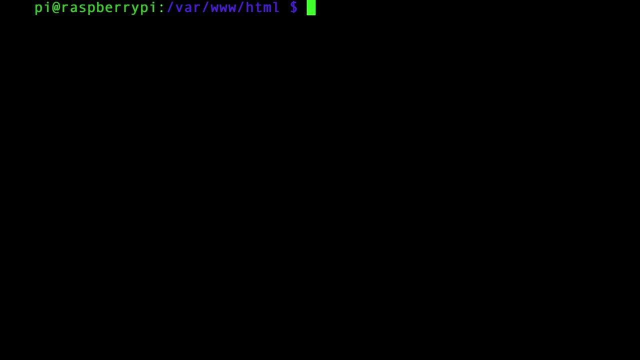 So, before we create our own HTML page and do fancy stuff, I want to own that HTML folder here, because I'm not the owner of it. Okay, As Pi the user, Okay. So what I want to do is go back a little bit and then I want to do a sudo chown, which 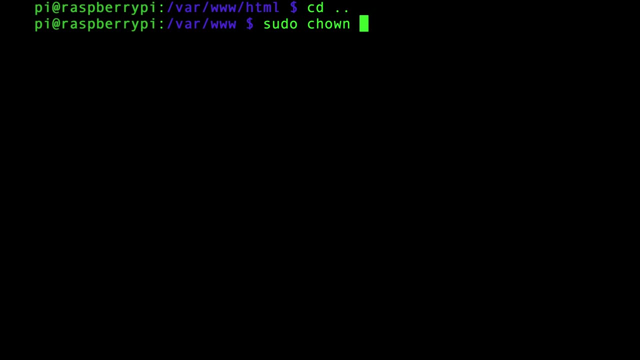 is change owner And chown this thing from Pi on this folder. Okay, So that means the owner of this is moi. Okay, Moi can now write stuff in it, because previously I couldn't. So the first thing I'm going to do, first order of business: remove this file. 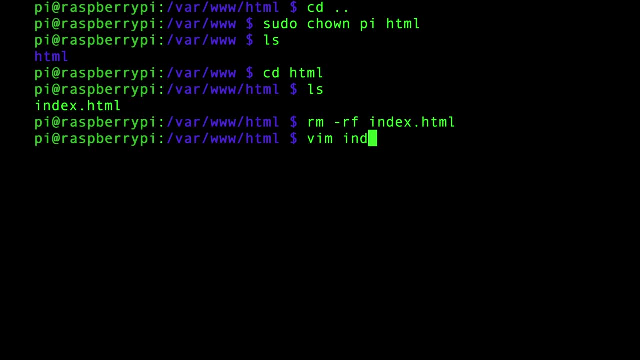 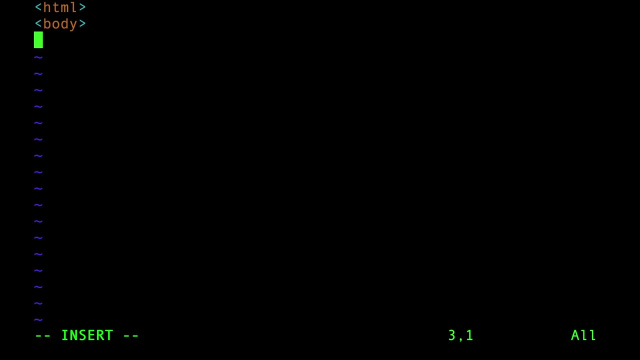 Okay, And I'm going to create one from scratch called indexhtml. Okay, And it's fancier. Okay, It's going to be fancier, I'm going to do hello world. This is my page, hosted on httpd or Apache 2, because the first version sucked. 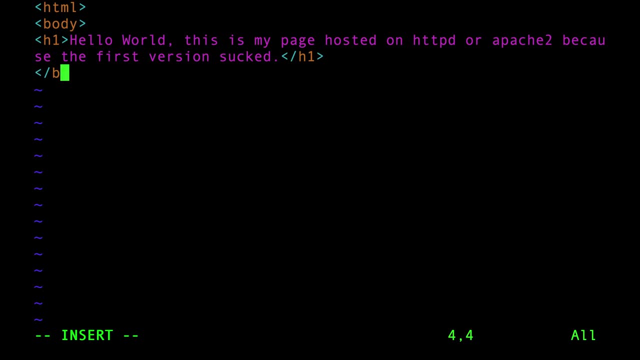 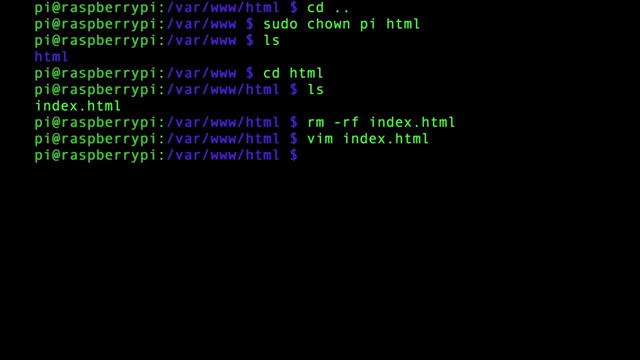 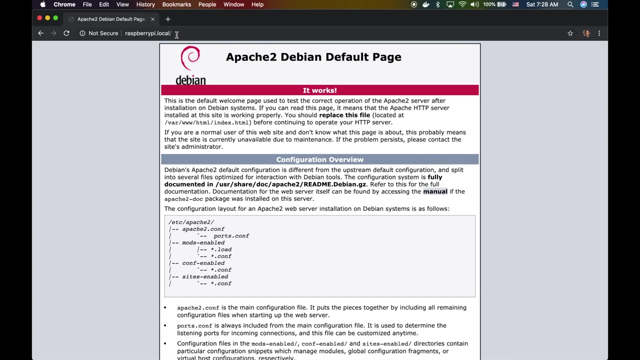 Okay, Buddy, Did we close that? Yes, we closed this, And then we do, and then that's it. We just created an indexhtml. Let's go back to my Mac. All right, We are in my Mac. I am about to hit refresh. 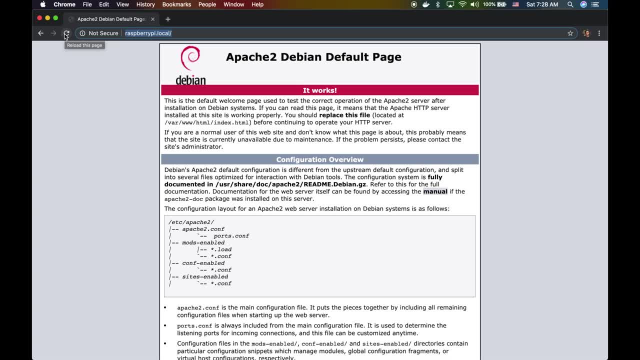 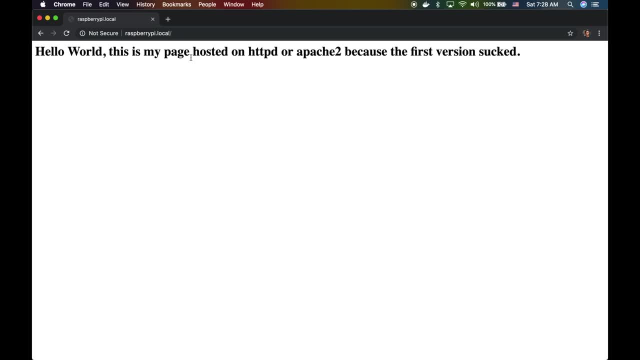 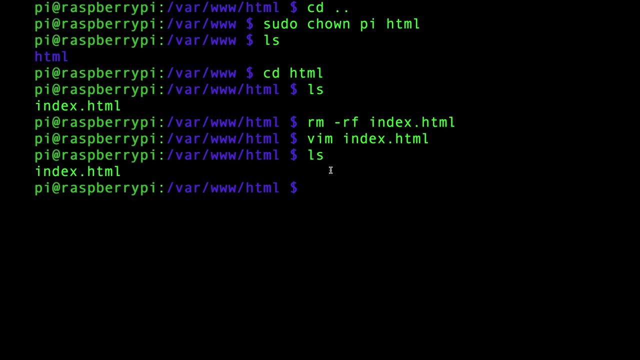 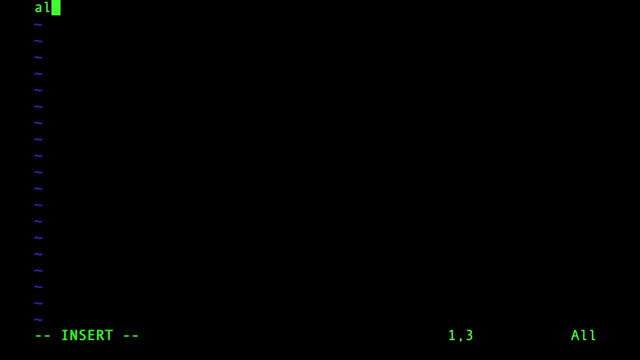 Hopefully my server is smart enough to not cache that page And guess what It worked. It worked All right And you can pretty much put any stuff there and it will just get hosted for you. Okay, And let's say for example, I don't know, let's do a mainjs file here and that does. 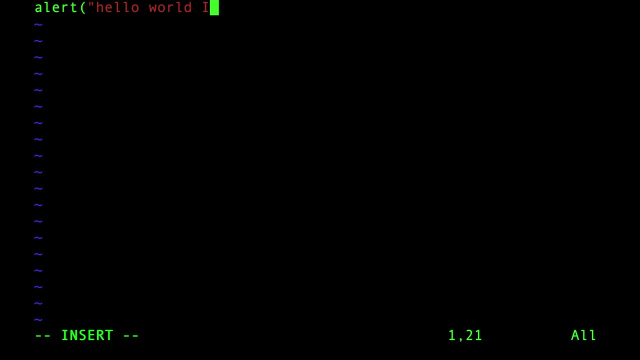 literally an alert. Hello world, I'm JS, Okay, And then we can edit my indexhtml and then we can do fancy stuff like that here in the body saying script as source equal: Was it? Was it Mainjs? Since it's in the same folder, we can get away with that. 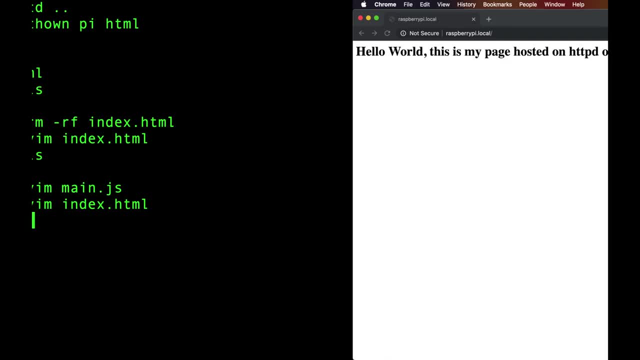 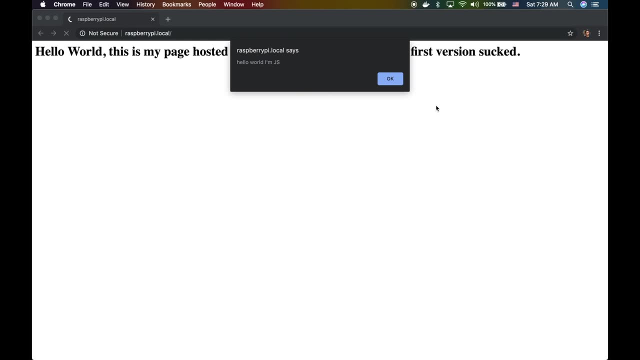 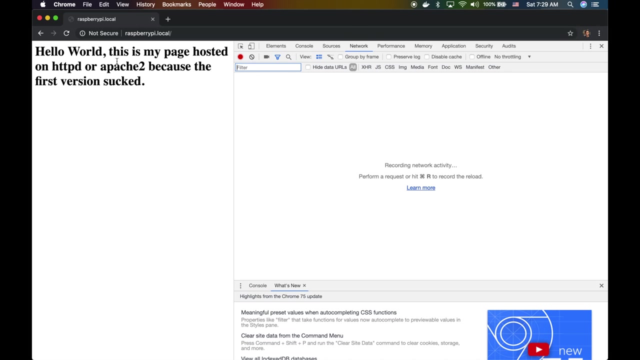 So let's do that. And then when we refresh, we're going to get an alert because my JavaScript got executed. So what happened here? if you literally took a look of that, right, When you refresh, two requests made right. 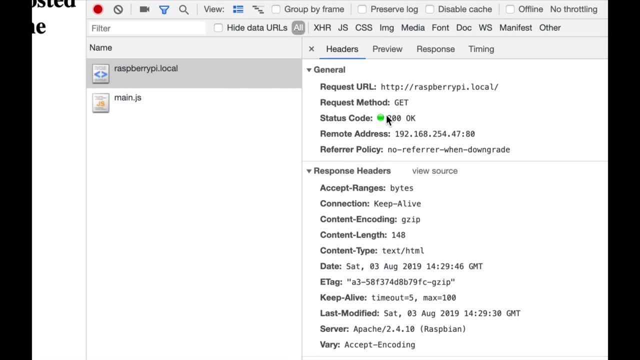 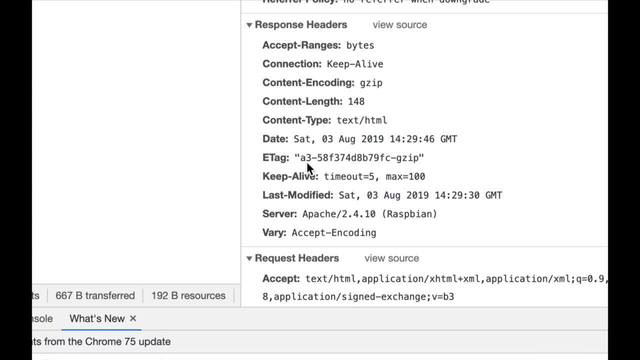 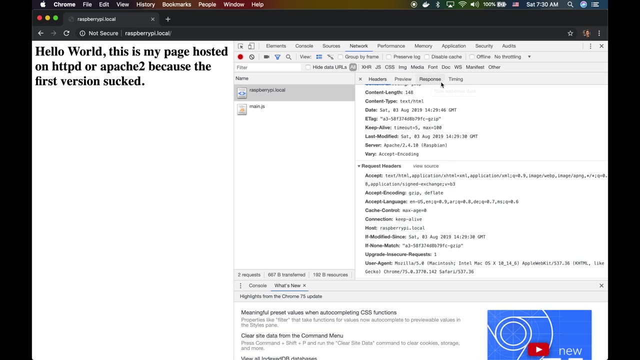 The first request is to get the indexhtml. This is the 200.. Okay, Obviously, we talked about that. We go back and indexhtml. It's a text right And that thing, when parsed by the browser, discovered that there is another thing it. 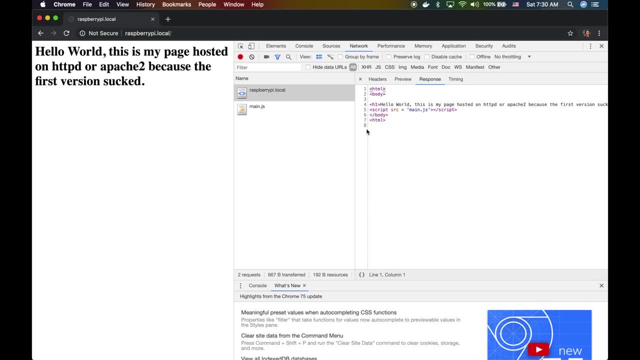 needs to pull. So that's back to our TCP connection thing, guys. So if HTTP 1.0, these two was two TCPs, We're going to have two TCP connections, which is extremely slow because every connection, every request will start the TCP connection and close it at the same time. 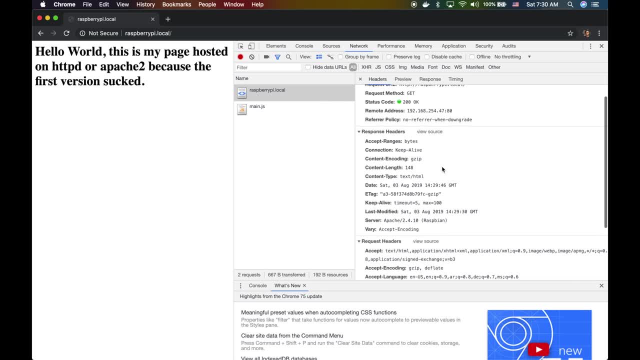 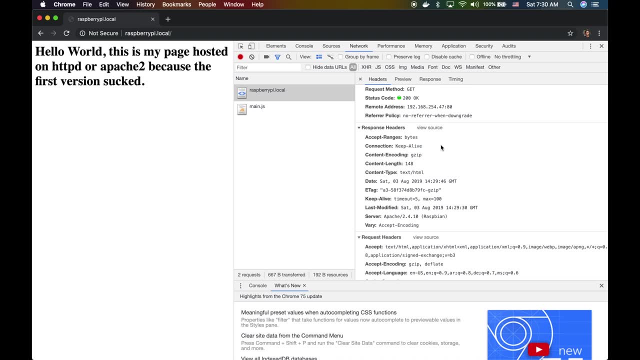 Now there's something called keep alive. I'm alive. Oh my God, this video is going to get demonetized. All right, Keep alive. right, So it's going to keep it alive. Keep the connection alive, baby. 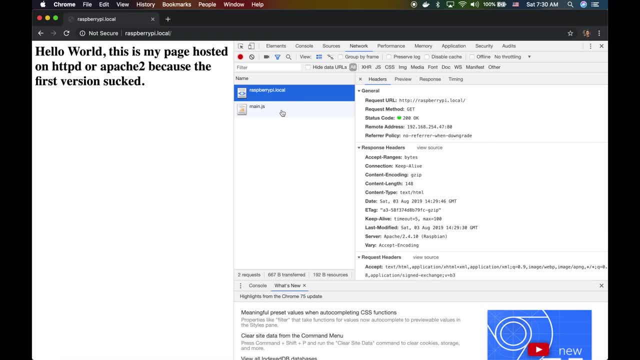 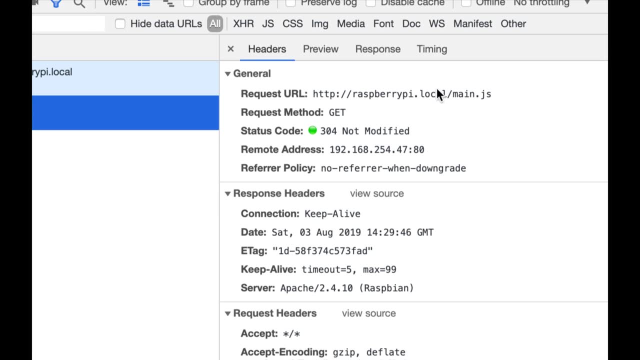 That's what it. Yeah, Keep the spark alive. So once it keeps the connection alive. the second request: okay, will actually make that request. It will actually make that request to get that mainjs. okay, Obviously, when you write your own observer, you have to do all of that manually. 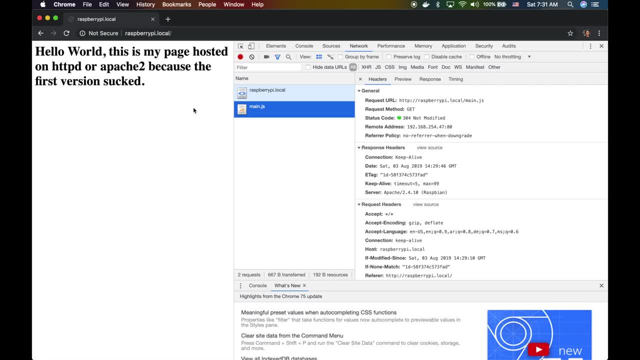 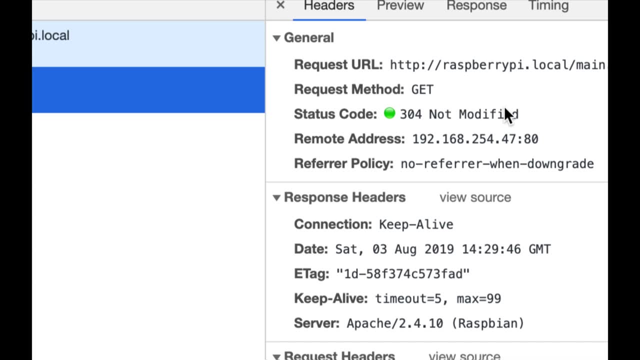 You have to do the caching manually, You have to do all that stuff, But this guy, Apache, does caching for you. okay, And let's prove it. So 304 not modified. that's the ETag. okay, Guys, I'm going to reference the ETag here. 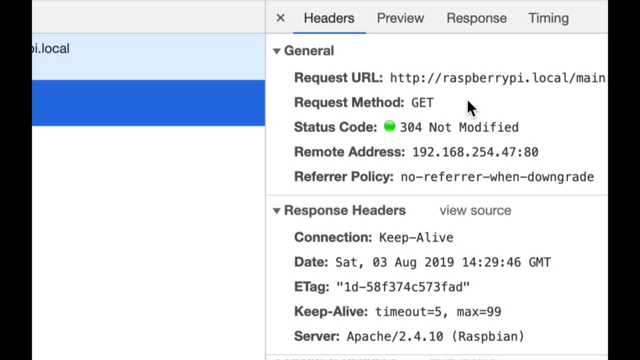 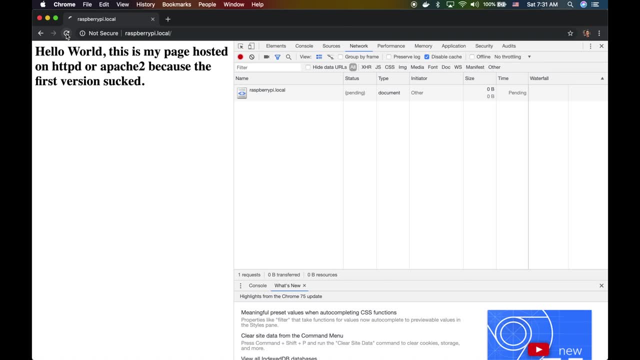 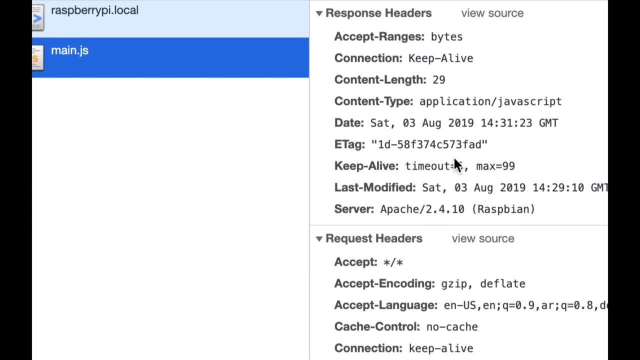 Go check it out. What is the concept of that? But in a nutshell, this is a caching mechanism. So the first thing, the first time, Let's disable caching. Let's show you that The first time I make a request okay to any content, I get back an ETag okay. 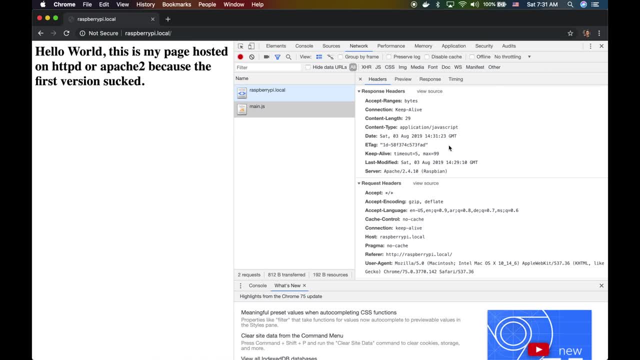 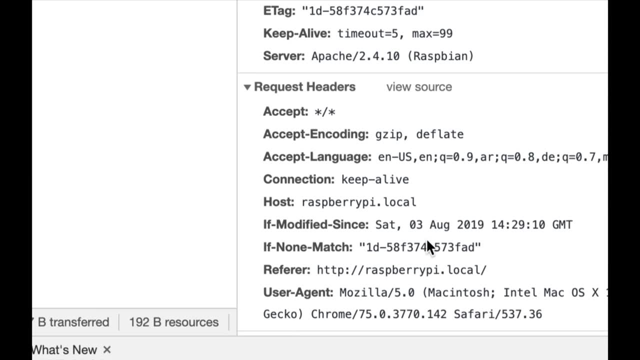 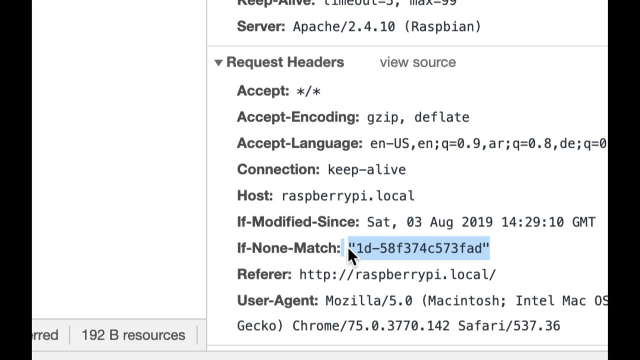 And the client then use that ETag with every single request it makes. okay, So if I make a request now and the client sends that request, says hey, if none match, tell me, Does ETag change? Tell me. 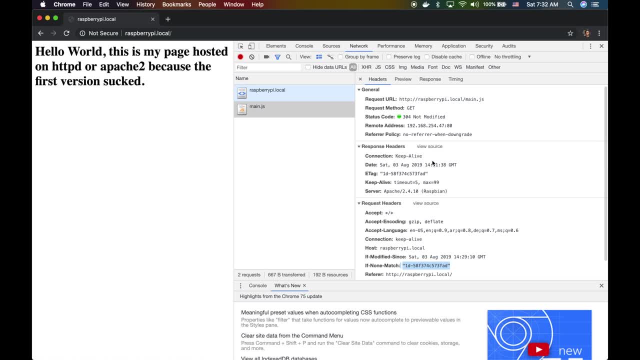 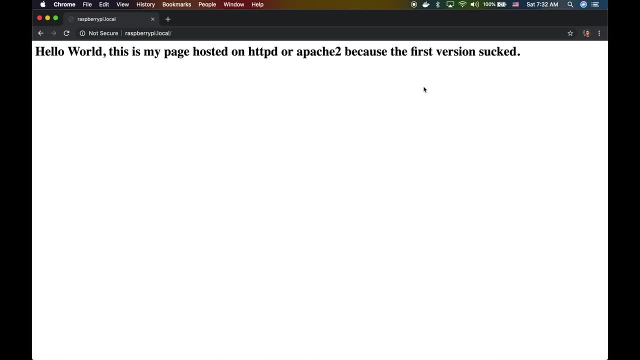 If it didn't change, coolish okay. But in this case the JavaScript didn't change, So it says: nah, you're good, Whatever you have is good, okay. So let's see how good the Apache implementation is. 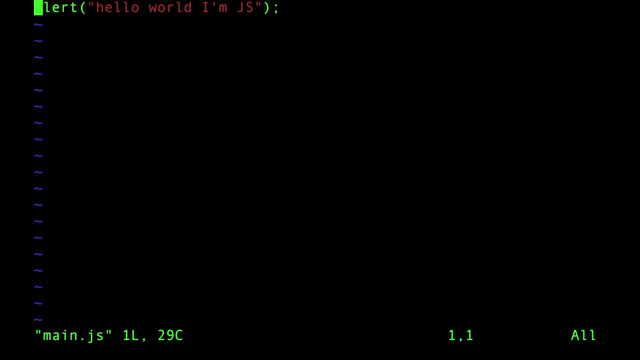 So I'm going to go ahead and do mainjs and I'm going to edit that thing to say alert, hello world, I am JS and I just changed baby. okay, And sure, let's do, I don't know. another alert message, because that's the only JavaScript. 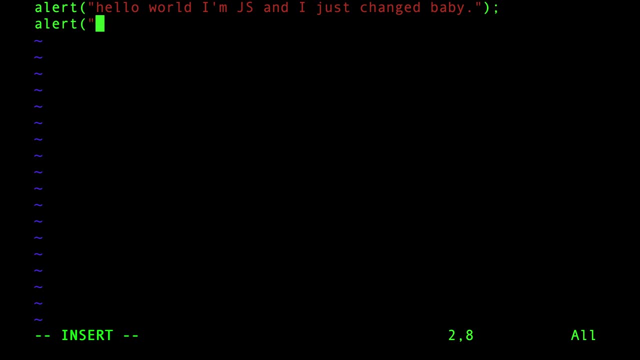 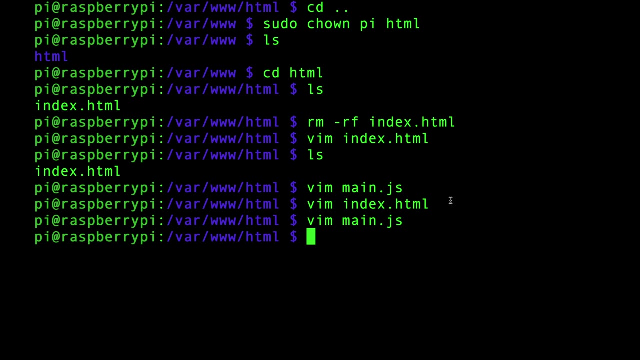 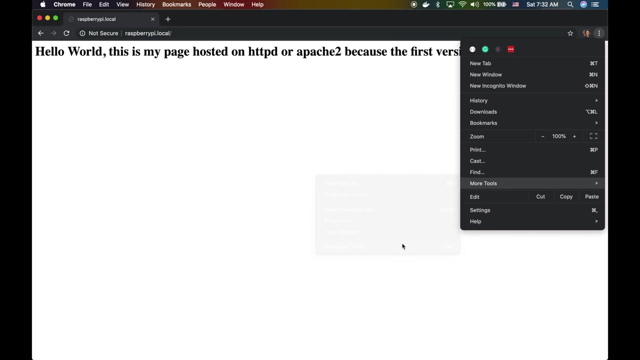 code. I know Kidding guys, I'm kidding. Oh my God. All right, That's another JS, right? Let's see if the implementation of the thingy is smart. So I'm going to go ahead. and What was our original? 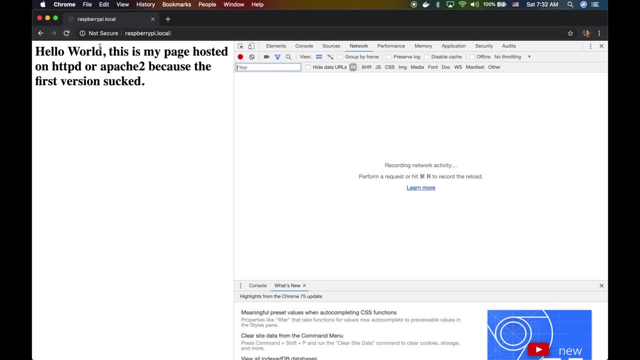 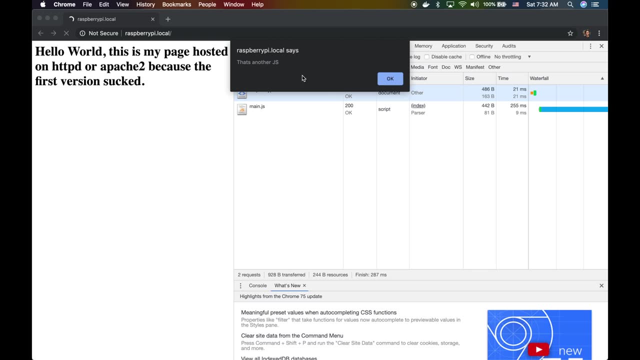 I lost it, Dosh. Okay, no problem, It was a certain ETag The client was trying to. The client will attempt to send the same ETag. but what, what, what, what? Look at that We got the new stuff. 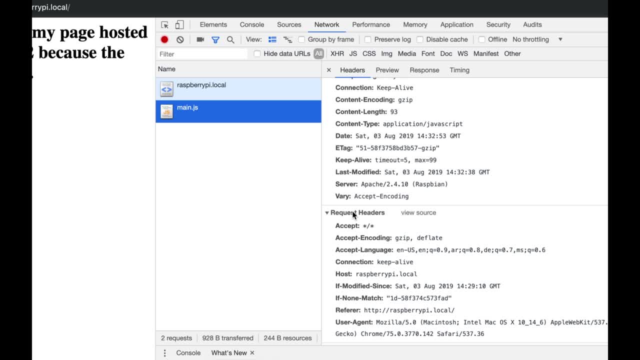 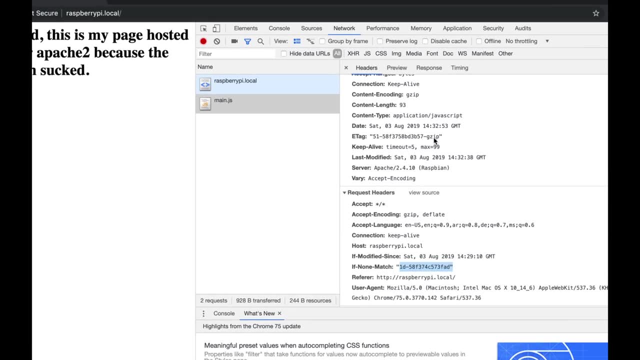 That's another JS, right? So what happened here is we sent it the same ETag, but we thought: nope, nope, nope, nope, nope, we got a new ETag. okay, I don't know what gzip is. 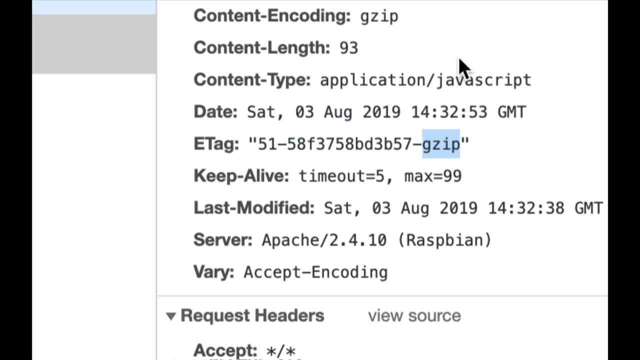 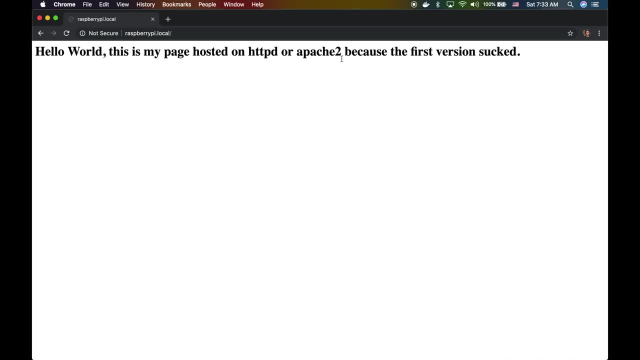 We're zipping this thing. That's wild. It's just like the implementation of the actual web server here. okay, So the web server says, nope, It has been modified All right. So that's essentially the trick, guys. 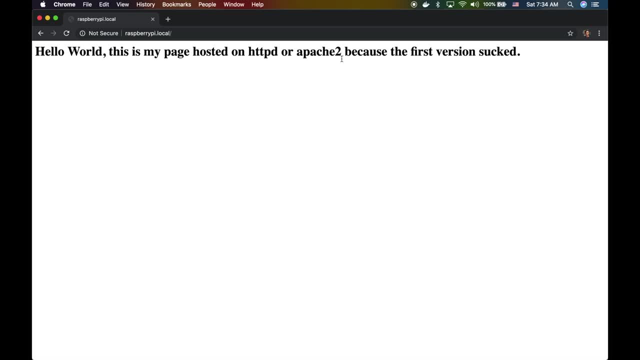 That's that simple stuff. Let's show you how Nodejs works. How about that? Right, So we're going to write our own implementation here. So, in order to write our own implementation, we need some decent editor. We cannot do use vim. 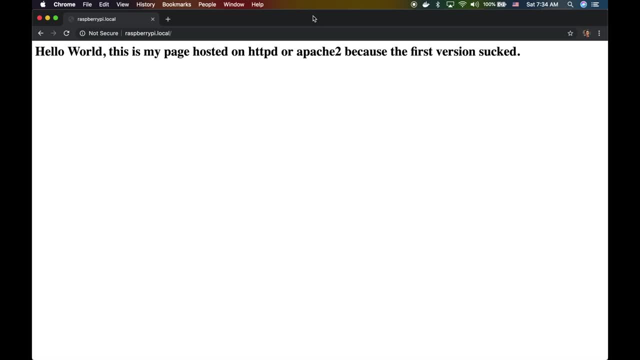 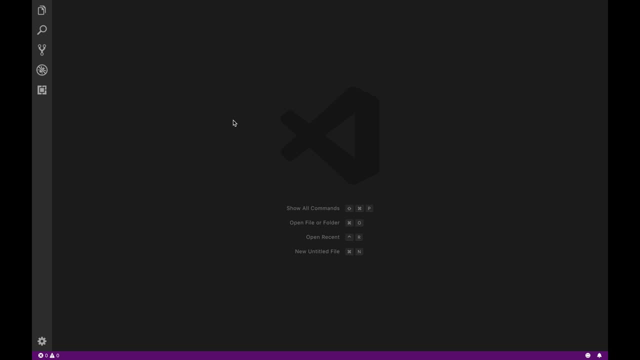 I mean we can, but yeah, It's just a lot of work, All right. All right, Let's show it here. I have Nodejs installed. Go ahead and check it out. I'm going to reference a video that we have installed with Nodejs and all that stuff. 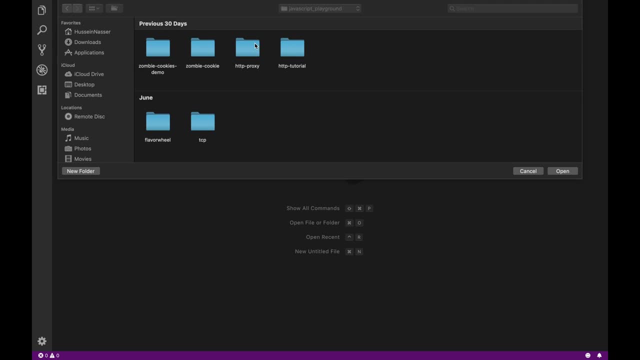 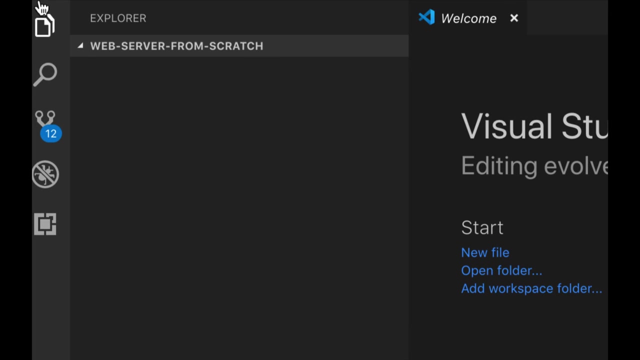 What I want to do essentially is just create a brand new folder with Visual Studio Code- Let's call this web server from scratch, okay. And then just a brand new folder. There's nothing in it, okay, And you go here and then you click on this guy and you will create a new folder. 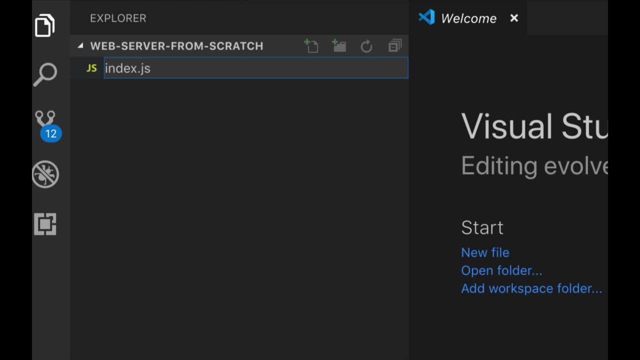 File And that file because I'm writing JavaScript on the back end. you have to write your own code here to do everything. okay, To serve a web content here. So I'm going to say indexjs and I'm going to create our indexgml page here. 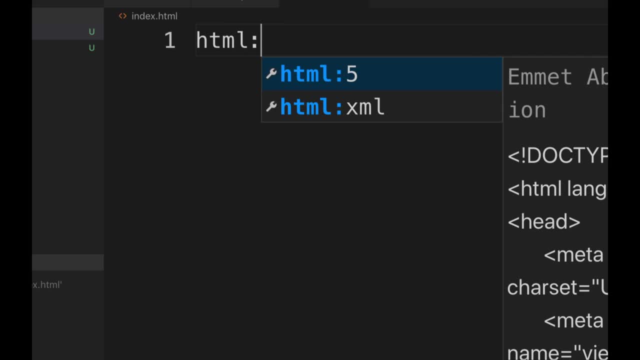 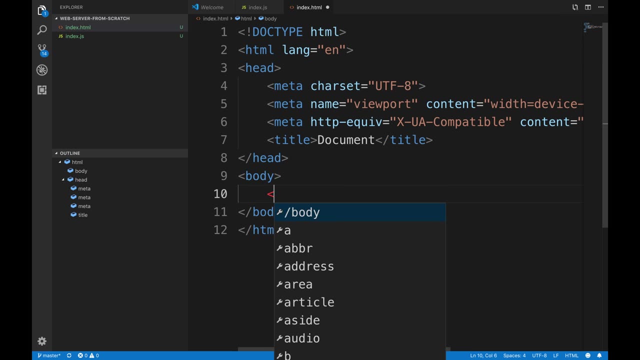 And since we are in the editor, we can actually write the entire HTML with just one click, instead of having to write everything. Hey, H1.. Hey, I wrote all of this myself, Nodejs babes. Okay, So that's the HTML that we want to serve. 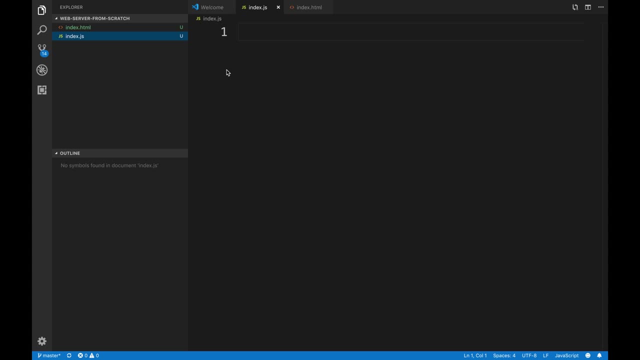 But we need to listen to a port, We need to receive requests, We need to send requests, We have to do all of that stuff. So let's get into it, guys, And you pick. then at the end of the video, you pick what is the favorite part for you. 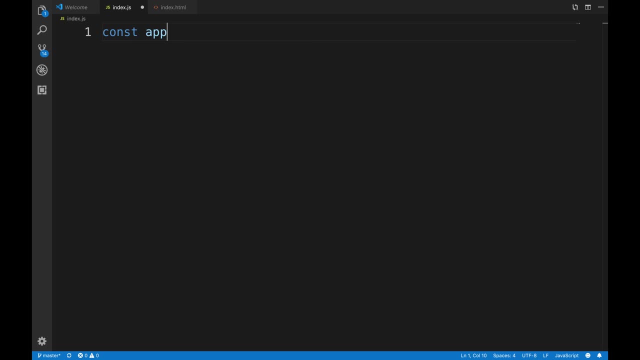 okay, So I'm going to do an app here: const, app, equal, require, express. okay, And that's just the bundle. So we need the app. We spin up a version of that. okay, Literally, a function call or constructor or tor. ctor. 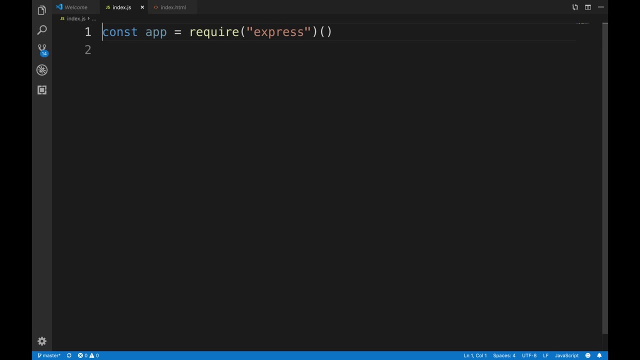 I don't know why everything is an abbreviation with people. okay, Constructor, Can't you say constructor? Really You have to type tor ctor. Oh, I know, man, I know you have people. guys, I'm telling you. 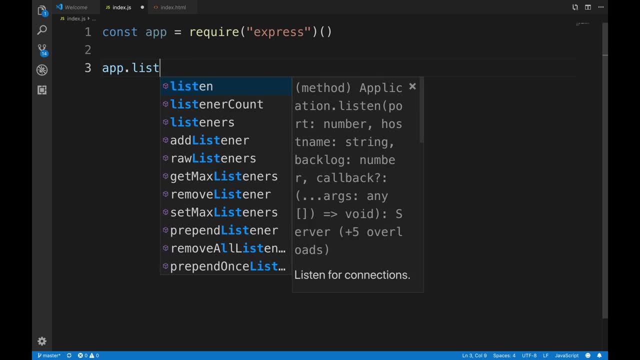 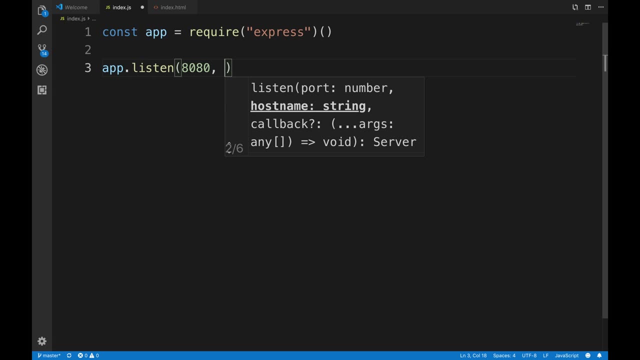 App. Here's what I'm going to do: Applisten. You're going to listen to port 8080, because 80 is kind of reserved for highly privileged apps and I'm not one of them, So I can't listen to them. 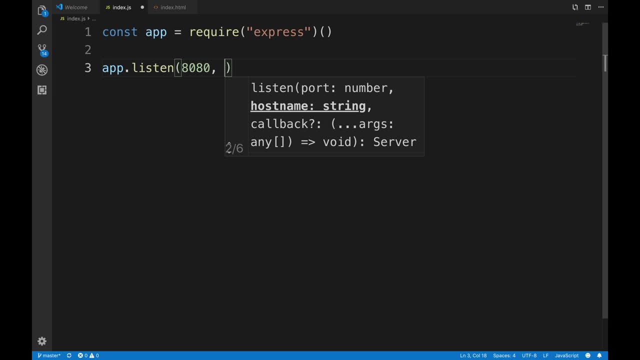 I have to run as a root and I don't want to. So let's just listen to 8080. And when you're done you say: consolelog: sup, I'm listening. Yes, What, What do you want? Okay, This is just for. 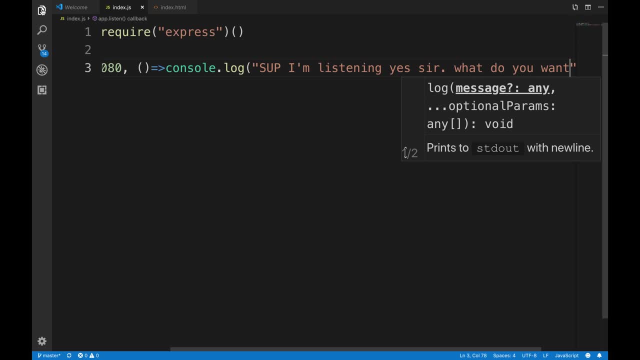 What the heck is happening. Okay, This is just for us to know that we're listening correctly, But that's not enough, Okay. Well, let's run it so we can show you. Okay, I have express installed globally, so that will work right. 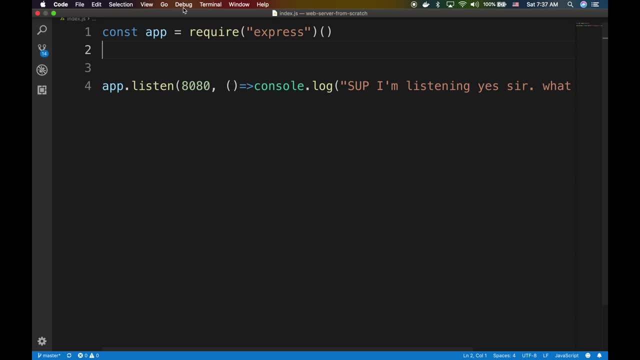 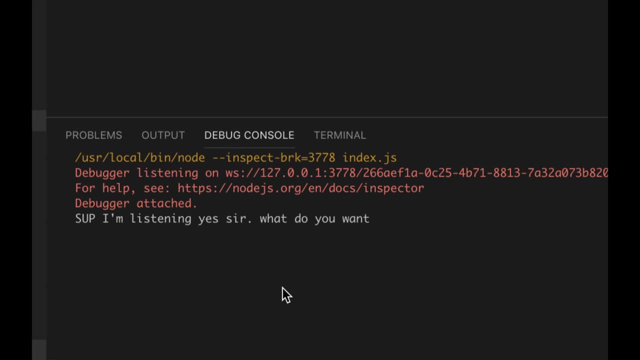 Well, that's it, Sup, I'm listening. Yes, sir, What do you want? Okay, That's it. Okay, But that's not enough, right? We need to really accept the request. That's If I do that. 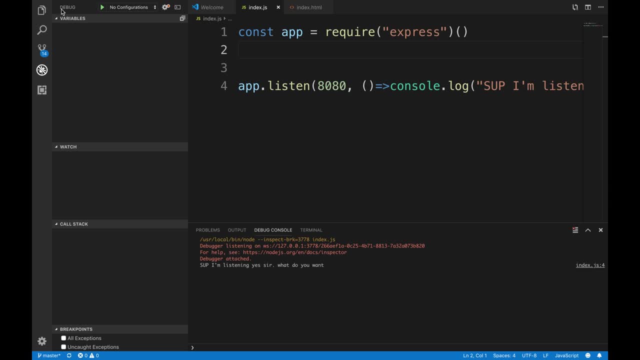 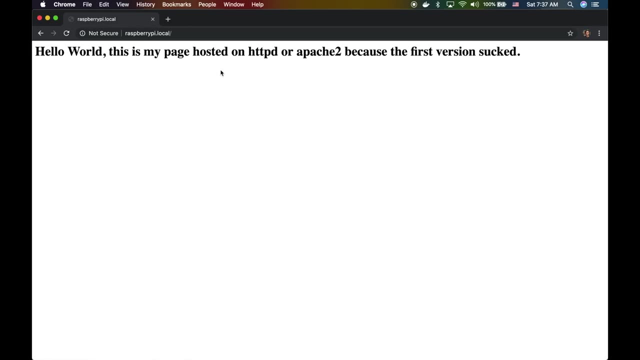 Okay, That's it, I'm listening. Yes, sir, What do you want? Okay, If I do that, now Let's see If I do that. and let's say run, let's just say localhost, right, See the error I'm getting. 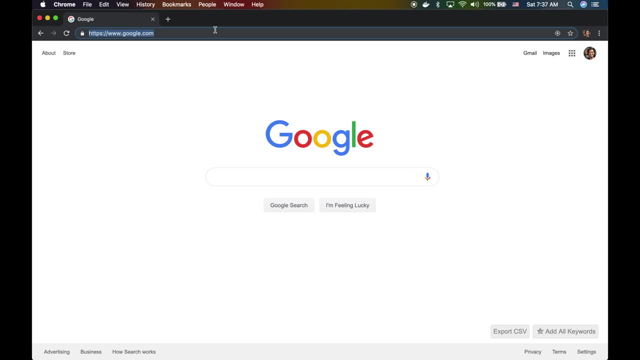 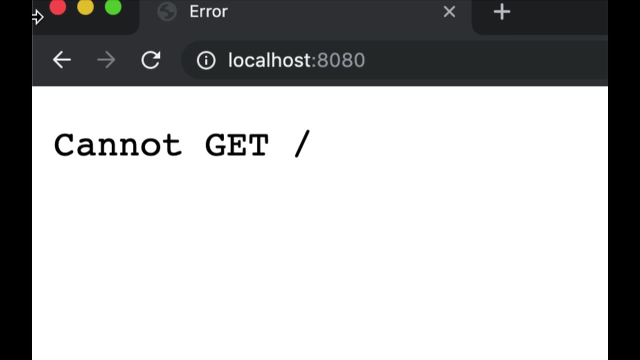 So now, guys, if I go and try to go to localhost, which is my machine 8080,, I'm getting this error. cannot get Why. Because you didn't implement anything right. There's nothing there, Okay. 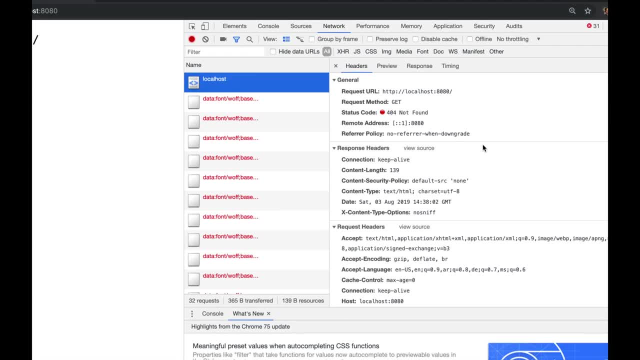 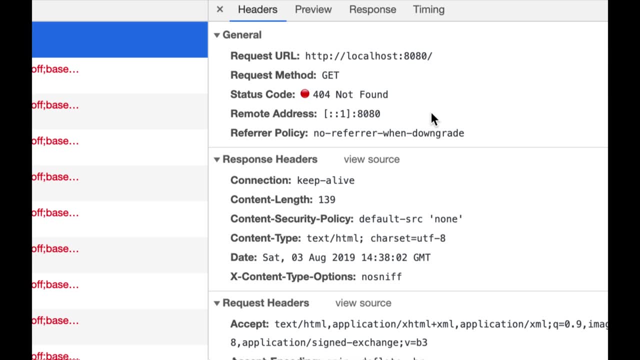 If you refresh there, look at all these errors, Forget about those. But look at that 404, because that's the only thing that the application does says hey, there's nothing on that server. The server is dead, Okay. 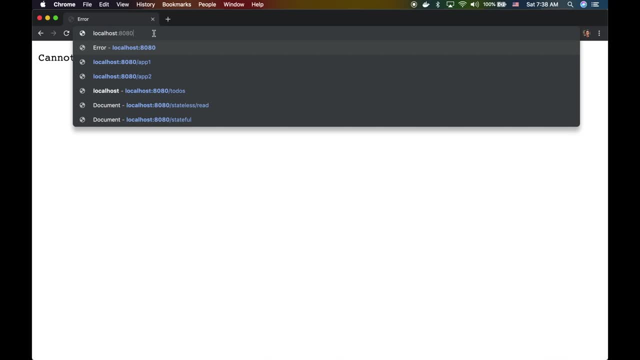 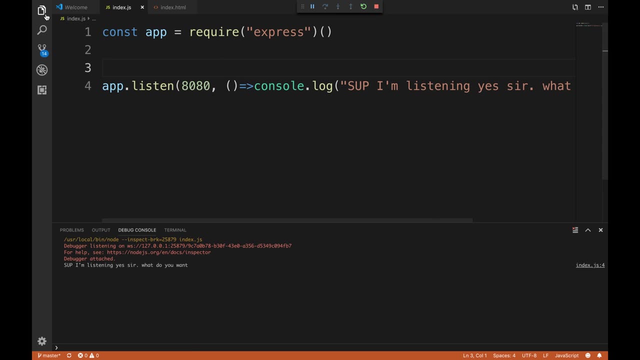 So here's what we need to implement. We need to implement a get method, a get slash method on the root, okay, So that's the first thing we need to implement. Remember, we didn't have to do any of that, Okay. 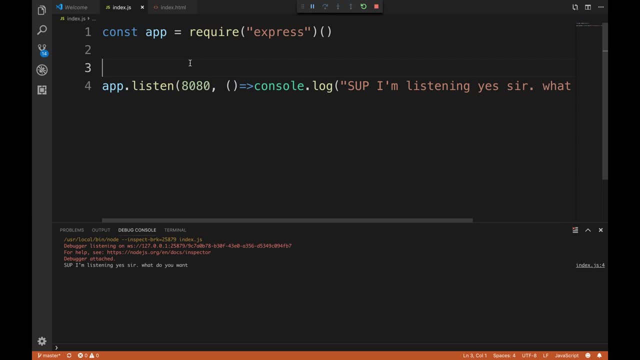 Well, we have an indexhtml. It didn't get served. We had to tell it to get served. How We can do apt or get On the slash. if someone visited me on the slash on the root, I want you to call this: 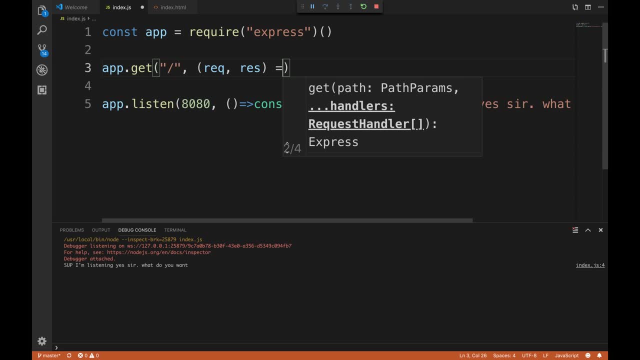 function, And this function always has to take two parameters: request and response. Okay, And then what you do, essentially for simplicity, is: you don't really care about the request. Sometimes you do, obviously, but here we don't. There's nothing in the request. 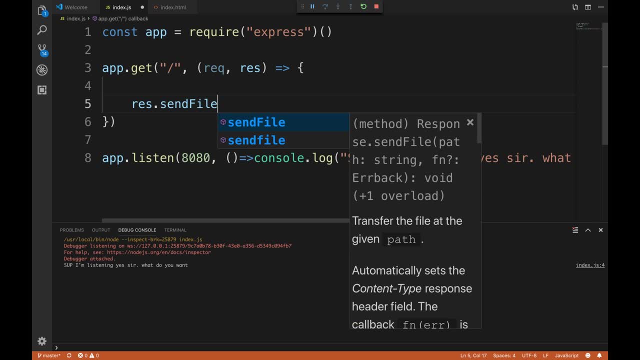 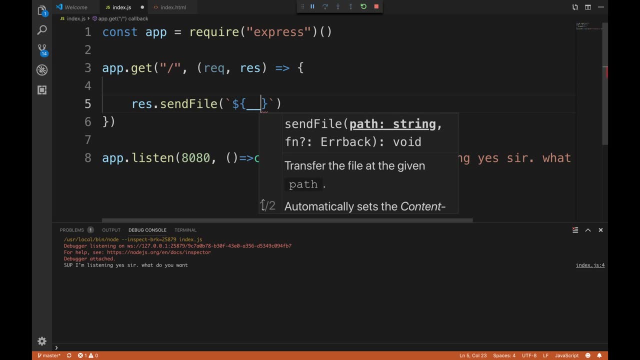 I just want, If someone visited me, I just want to send file and then you send it the indexhtml file. Okay, And to do that we have to do all that stuff where it's in my directory. This is to avoid hackers pulling over your stuff. 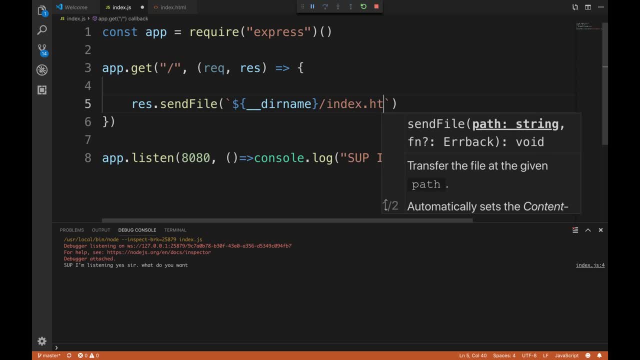 So you have to specify. You cannot use relative files here, So you have to do that. Okay, So that will take the directory name and then indexhtml. Okay, So that will serve the indexhtml page. Okay, Let's try this. 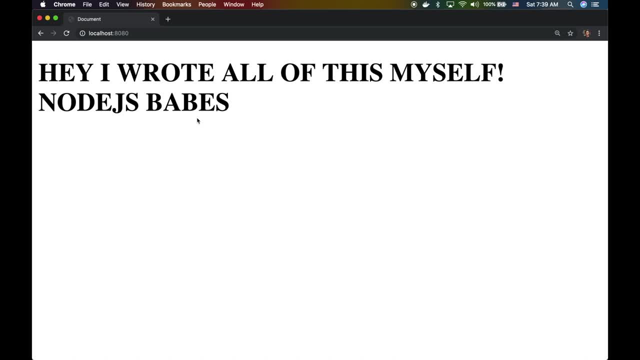 Restart. Okay, So if I refresh, Hey, I wrote all of this myself, Nodejs, babes, Okay, You like this. babes, You like it. This is the best. Right, This is the best, And if you've served another file, you have to do the same thing again. 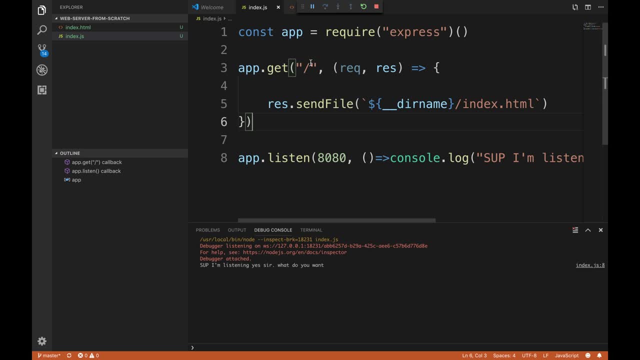 Okay, Anything. Okay. There's obviously regular expressions that you have, like any. If someone visited anything, then serve them anything A little bit dangerous. but you have to know what you're doing. But that's essentially it. That's essentially how you write web content. 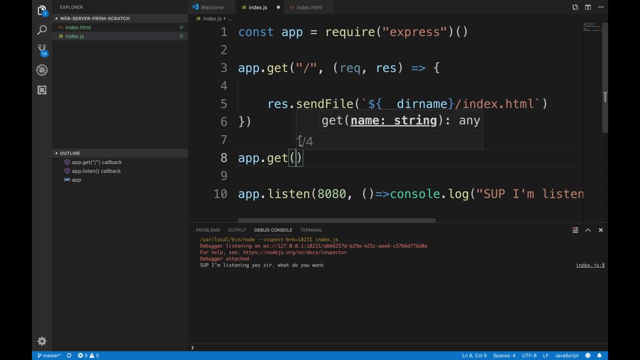 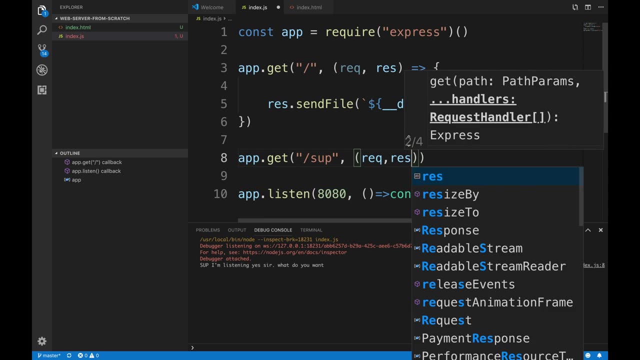 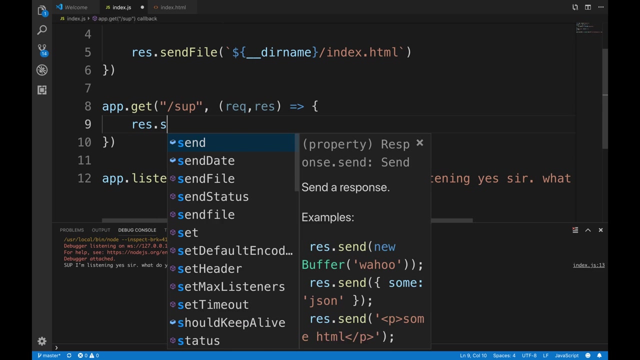 Can you do something else? Sure sir, You can do. get slash, sup, anything you want really. Then request response: You can do, And we have the function here. We can, for example, just send a result, Anything we want. 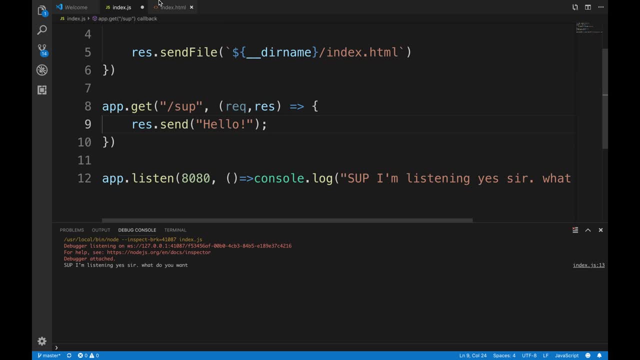 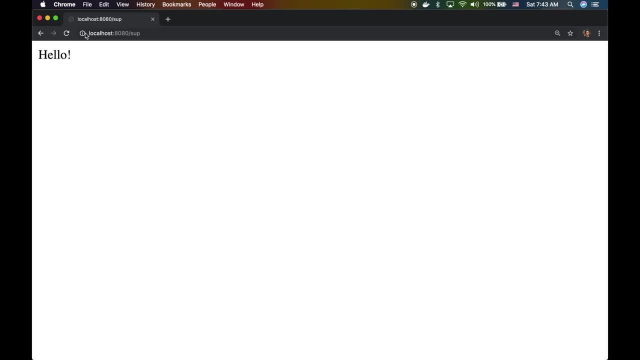 Text: Hello. Okay, And then if I do that, all right, if I go to localhost 8080, I get this. If I do sup, I get hello. And let's see what did we get back from the headers. 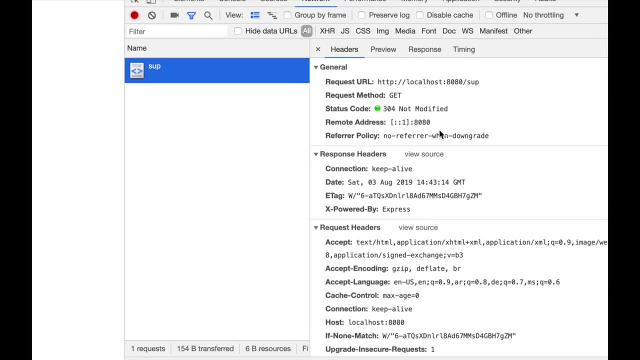 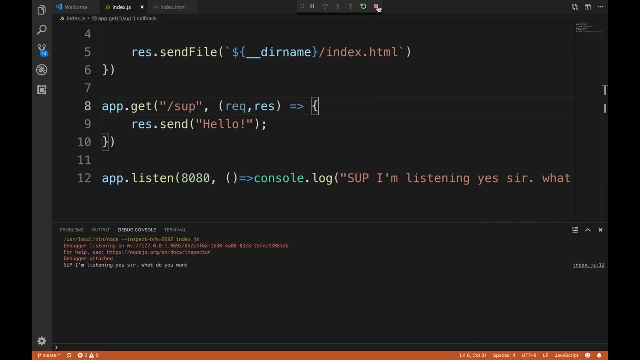 What did we get back from the headers? We get back 304, not modified, and we got back the results. Okay, And now can I change that? Yeah, sure you can. You can do resultstatuscode and instead of 304, you can change it to anything. 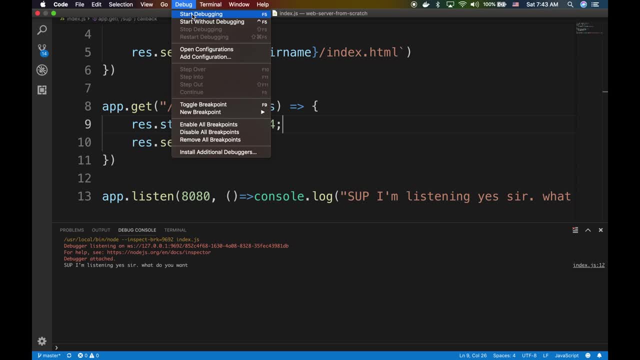 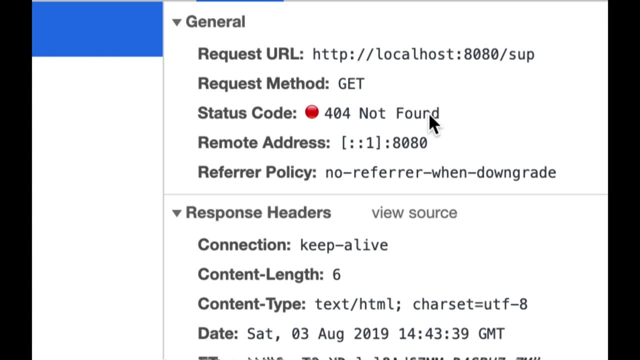 404.. 404.. What is a 404?? You guys know right. 404 is not found, although it was found, but you can tell it whatever you want. That's the flexibility you get when you write your own web server.